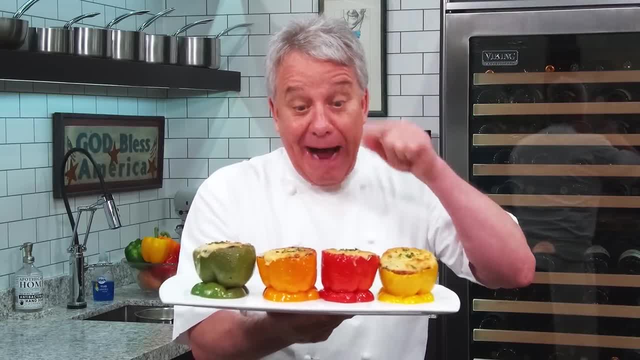 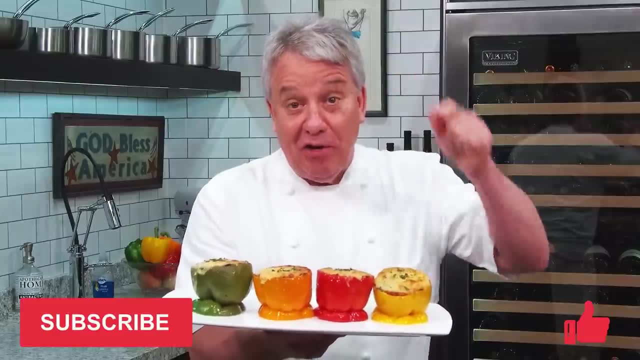 Well, hello there friends. Amazing recipe: today I'm going to make stuffed bell peppers. Wait until you see how easy it is to make. Remember: thumbs up. if you like the recipe, subscribe to the channel and ring that bell. Stay tuned, We're making them right now. 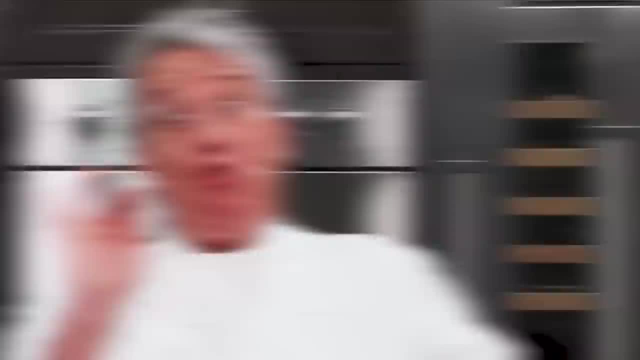 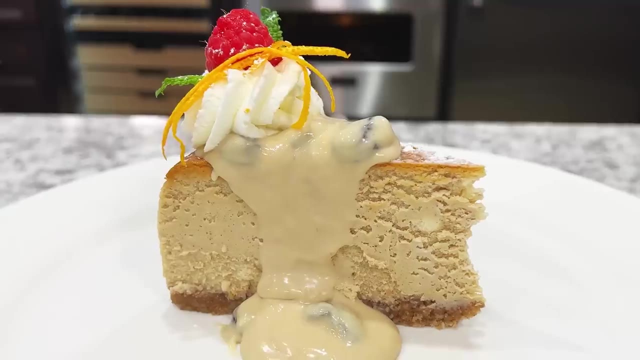 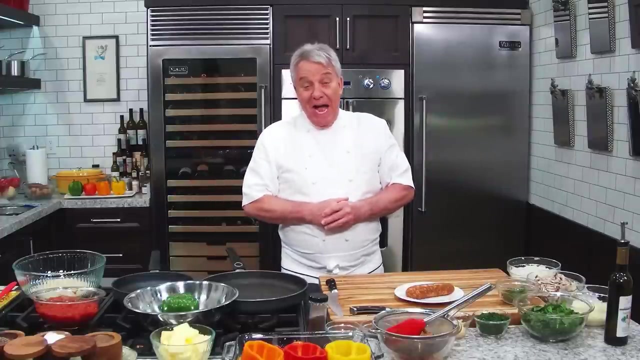 Okay there friends. Well, let me show you how easy it is to make those stuffed bell peppers. Actually, it's quite a lot of prep. There's a lot of stuff going on over there, but I'm going to show you It's going to be delicious. 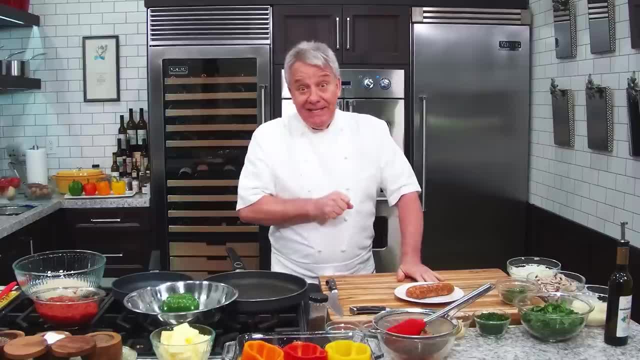 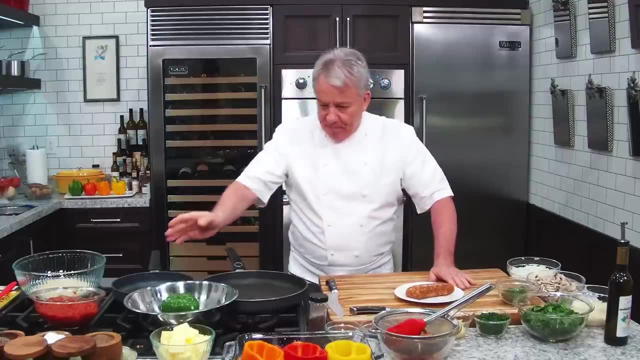 And the cool part about this, you can make them in advance. You can make two or three eggs while you eat them tomorrow for lunch. They're delicious. All right, Friends. I got all kind of peppers. I got sausages. 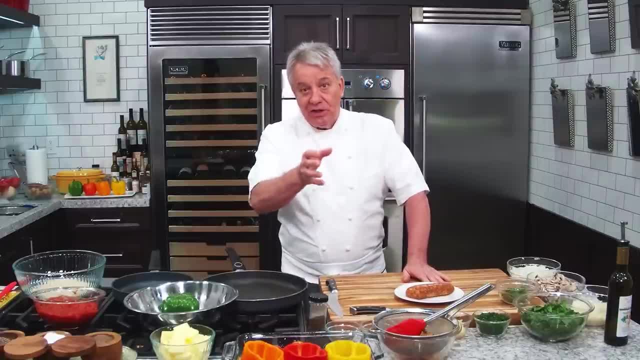 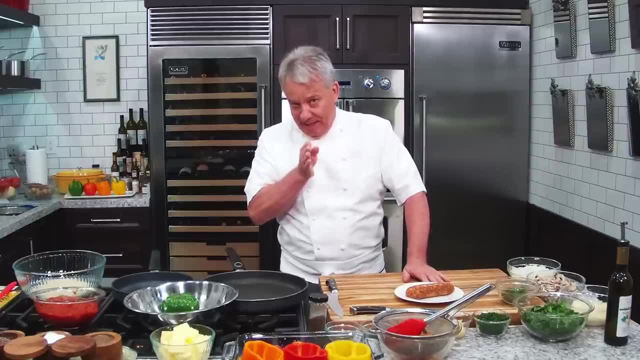 I got, mama mia, I got all this kind of stuff. You can stuff them with a ground beef, but I like better a spicy Italian sausage. I don't know if you ever tried it, but let me tell you it's amazing. 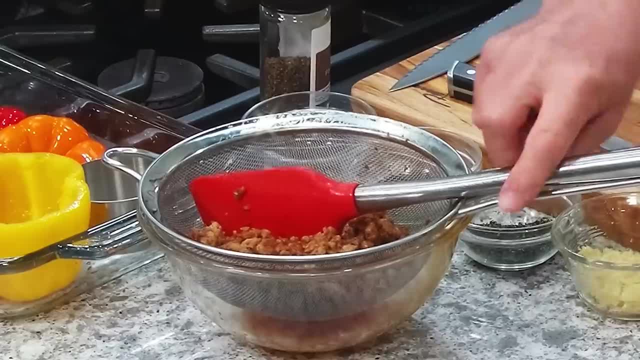 All right. So I got the sausage right here. I already did some of it, See, look, Look, I got it right there. Look, how beautiful that is, friends. Let me see. I hope the camera can see it Right there. 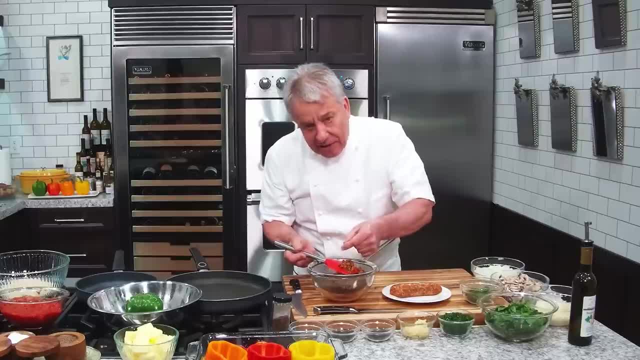 You see, look how beautiful golden brown it is. All right, That's the Maillard reaction. We're going to do that. I'm going to show you how to do it. See, and I got a little bit of oil. 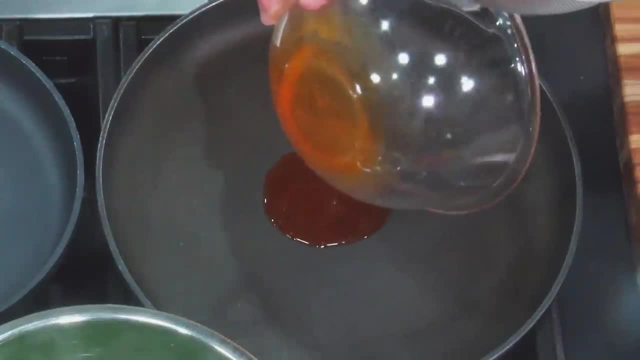 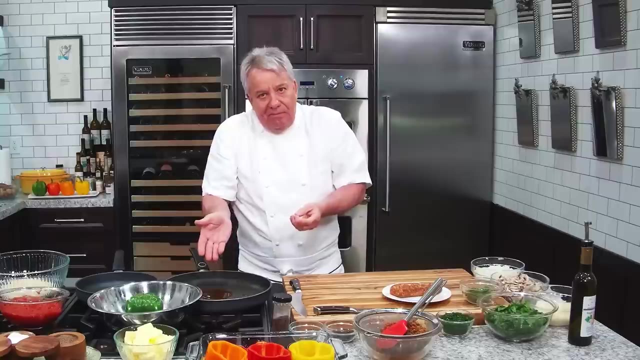 I'm dripping it and I'm going to use that oil right there to saute my onion. I'm going to use them instead of putting olive oil, which would be delicious, but I got this phenomenal oil, so I'm going to use it right. 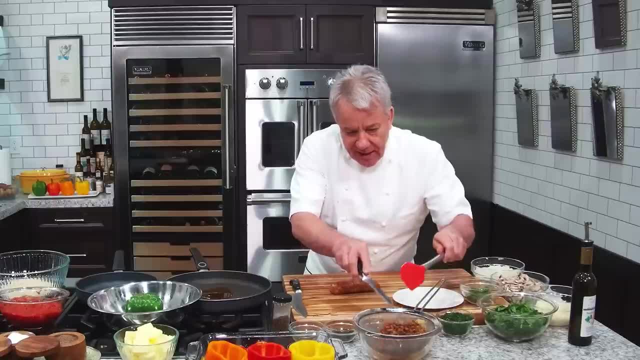 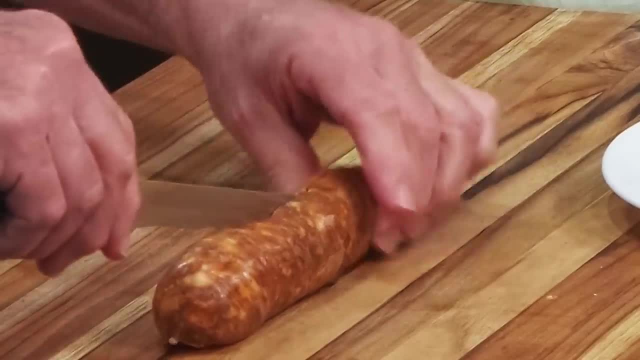 I want to show you how to get this into this. All right, I know a lot of you know, but I'm going to show you anyway. We're going to cut the casing off. okay, When you get the sausage, you take it, you cut it and then you take the casing. 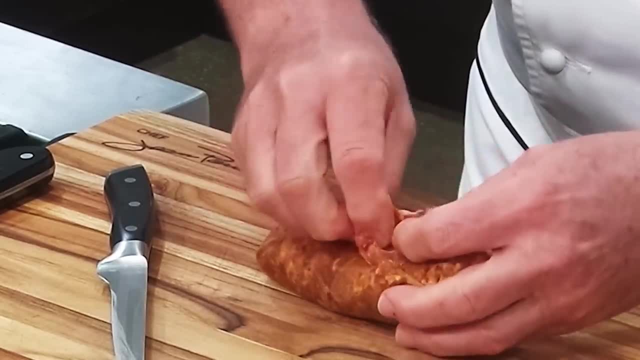 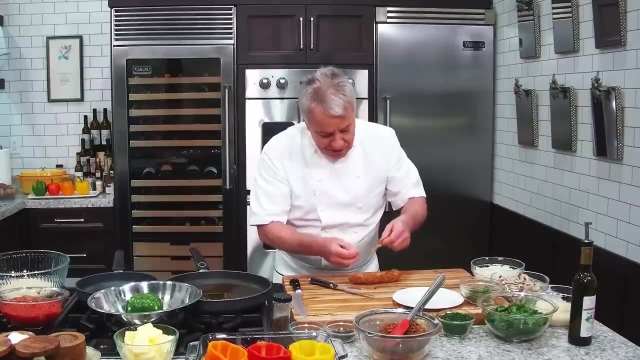 and you just flip it back. Normally it comes out really easy, unless there's camera rolling. then it makes it difficult for you. So don't do it with the camera rolling, okay, You take it right there, your sausage without the casing, okay. 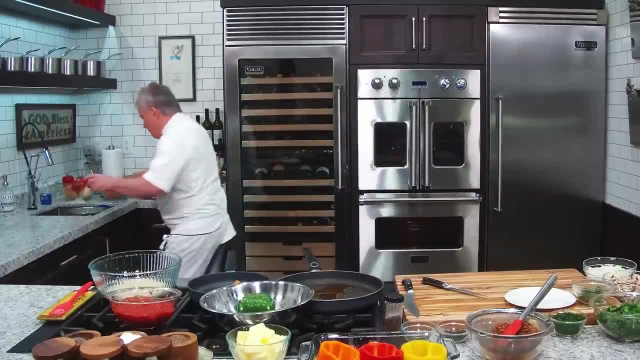 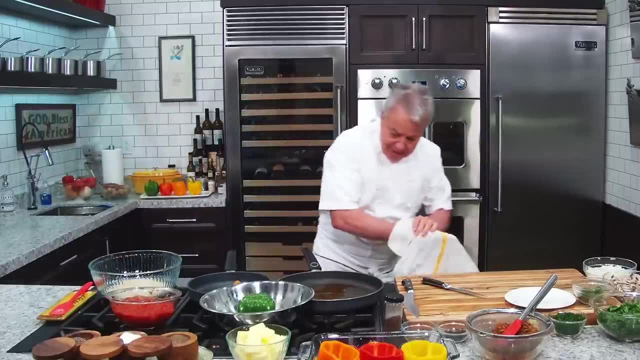 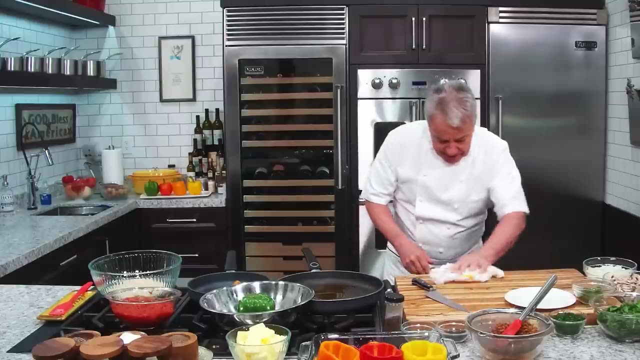 And you clean your hands and I'm going to show you okay. Okay, so let me just clean my hands, Let me take a sanitized rack so I can clean my board, clean my knife and I'm ready for the next step. 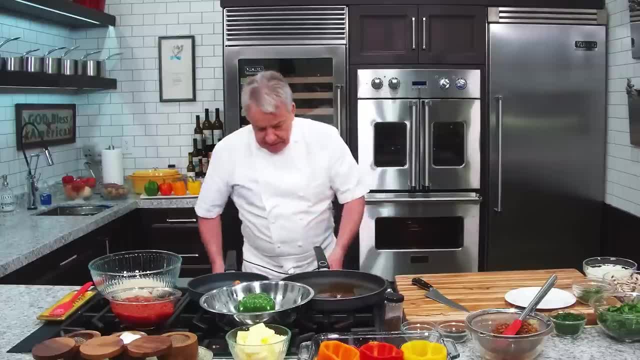 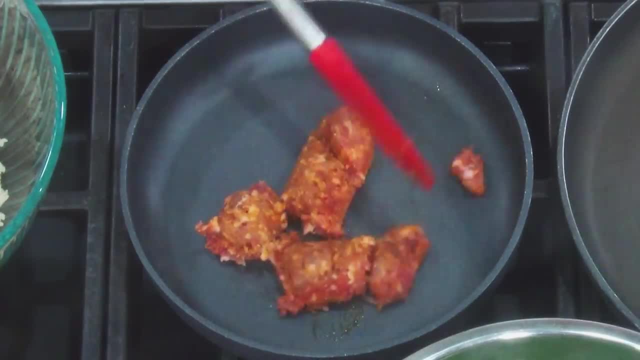 I got a lot of stuff to do, So this is it's not complicated, if you will. It's just a little time-consuming, but it's not complicated to do. You can do it, Anybody can do it okay. 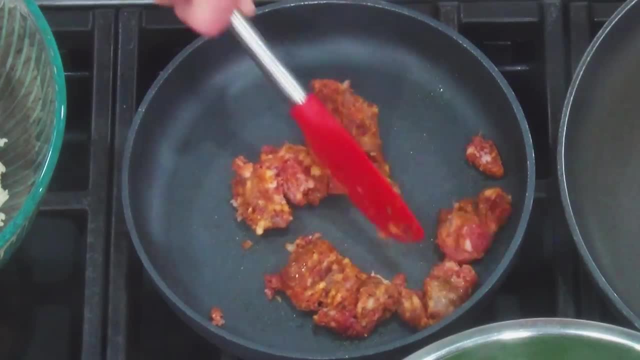 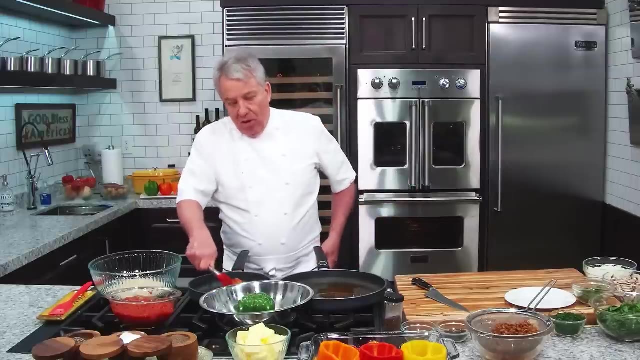 You know, I know some people say: oh, I can't do it, I can't, I can't cook. Well, guess what? If you never took any tennis lesson, would you be a good tennis player? No, If you never took any golf lesson, would you be a good golf pro? 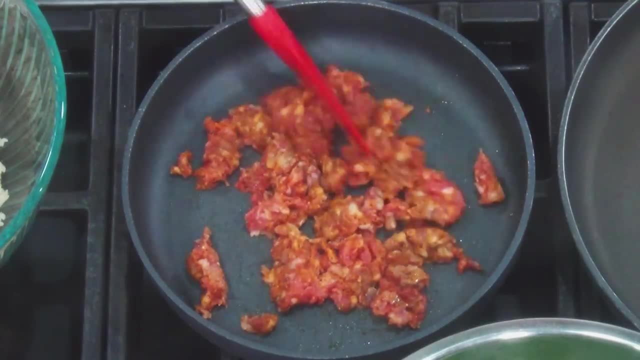 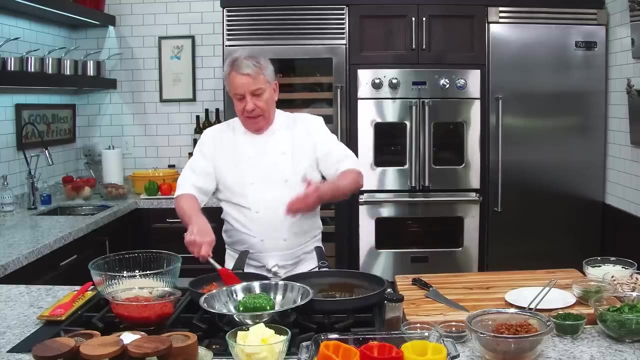 No, You take lesson, You learn. You're not born a good piano player, or you're not born a good tennis player or a good. you're not born anything. I mean you're born. Some people, right, Some people are talented. 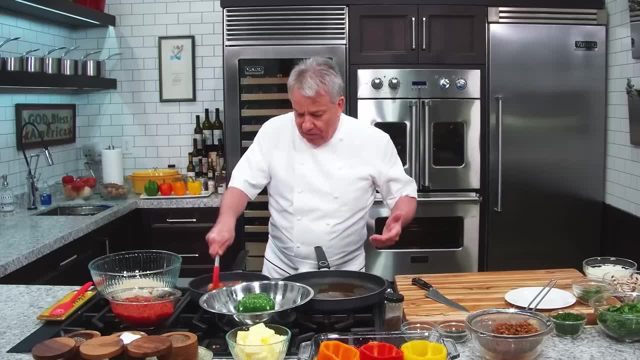 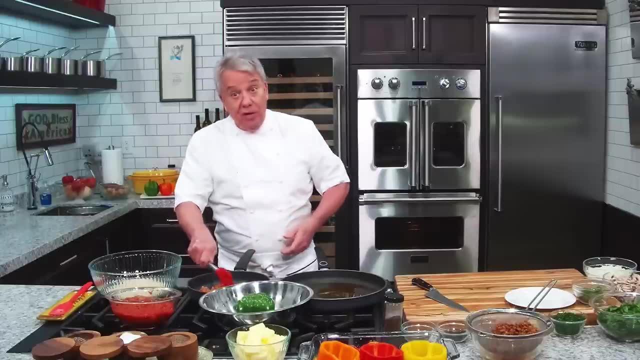 I was not one of them. I learned My mom was a call-in blue chef, so I was lucky to learn. I went next to my mom and then I studied. I did like 10 years of apprenticeship, So you got to study. 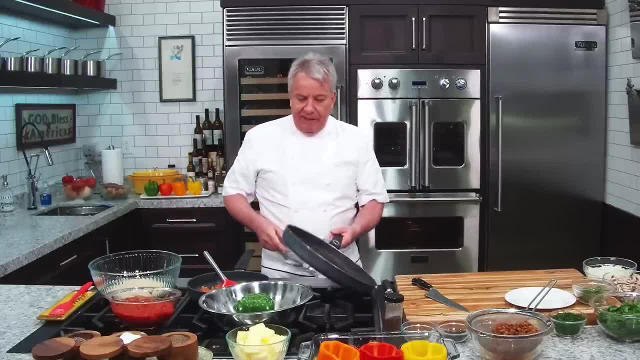 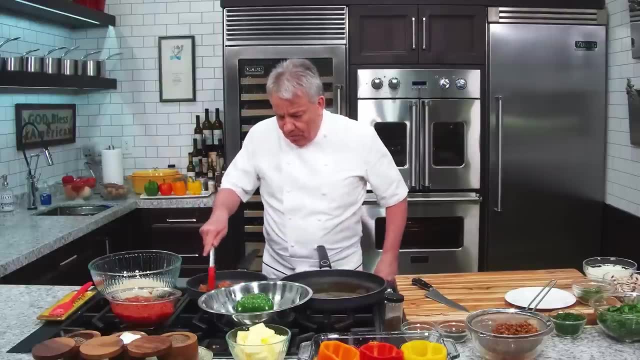 At home. the good part of it is you don't need to do 10 years of apprenticeship. You can be a really good cook really quick at home. all right, So and I'm going to show you. All right, That's the whole plan. 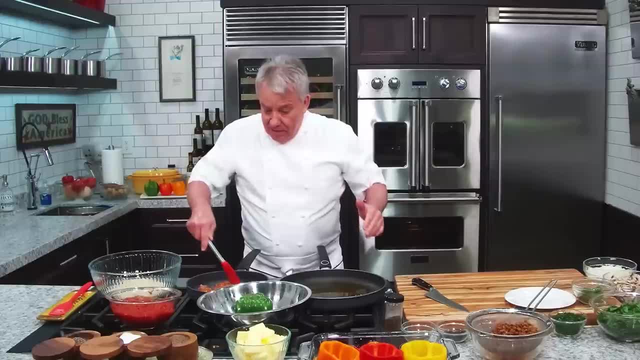 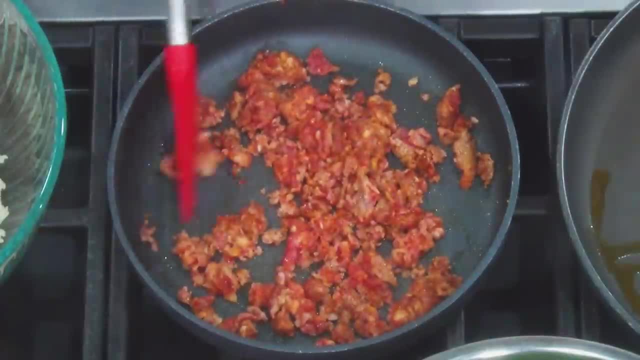 That's the whole idea is: anybody can do this. You can take your cooking from this to this in no time at all, because it's not complicated. okay, I don't think it's complicated. Take the sausage right there, break it up, do this, okay. 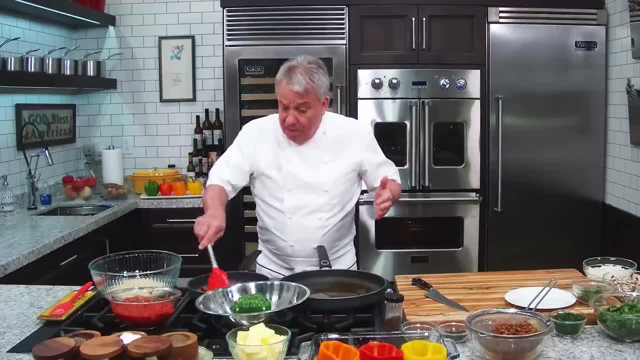 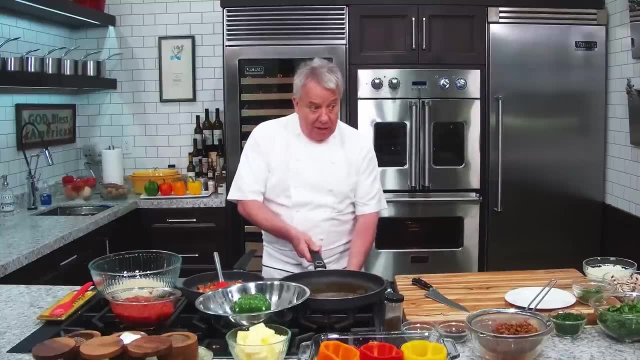 Buy you a good sausage, though You know that's the thing. You know you're going to be only as good as the product you use. You use good product. you're going to make good food. You use crappy product. good luck making good food. 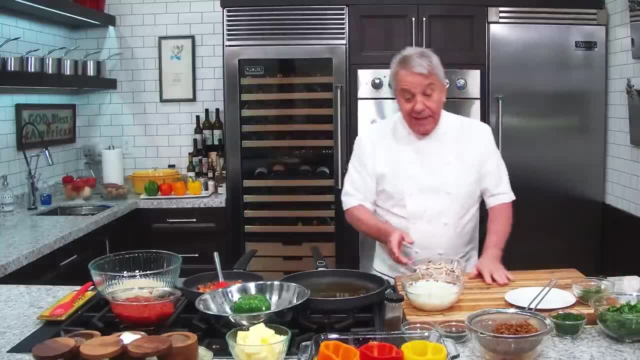 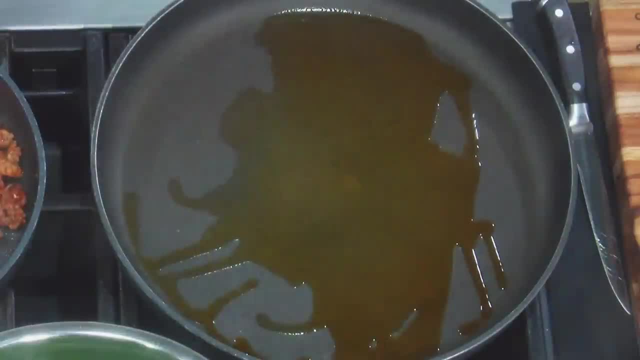 We're going to saute some onion. At the end of the day, you're only as good as the product you're using. All right, That's really that simple. So we got the sausage over there, We're going to wait until it's hot, and then you know what we're going to do, friends. 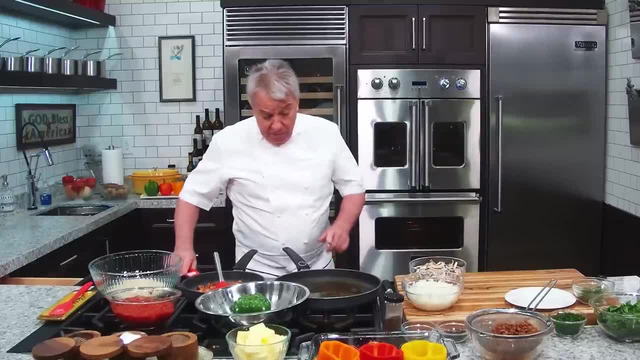 We're going to prepare the pizza. We're going to prepare the pizza. I'm going to show you what to do with the pepper. Well, I'm waiting. I'm not waiting that long, because I'm already at 320, and I need to be at 365.. 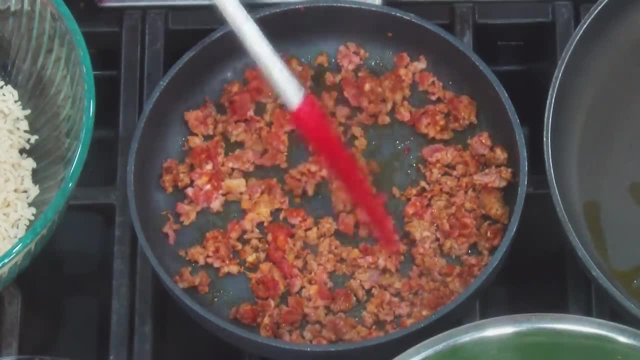 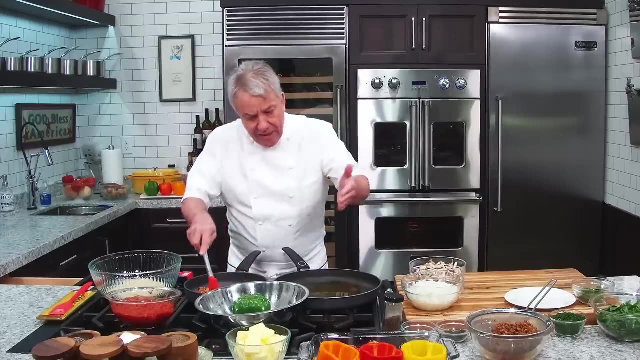 So let's kind of look at what we got here. We got the sausage is starting to get the Maya reaction, which is the most important. You see a lot of restaurants. sometimes you go and get a bolognese or something with a sausage like that. 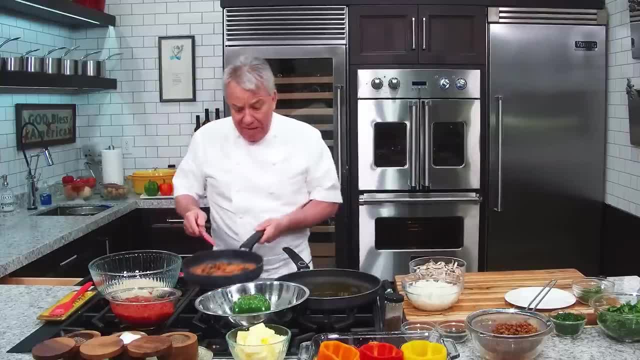 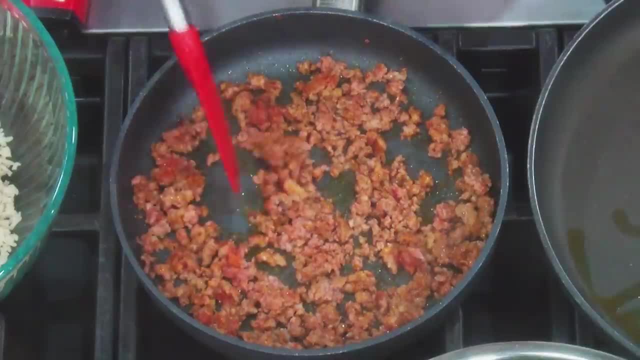 and you know what they do. They take this right there, they put it on the cutting board and they chop it up with a knife. Don't do that. Don't do that. You need the, The cronny. what do you call them? 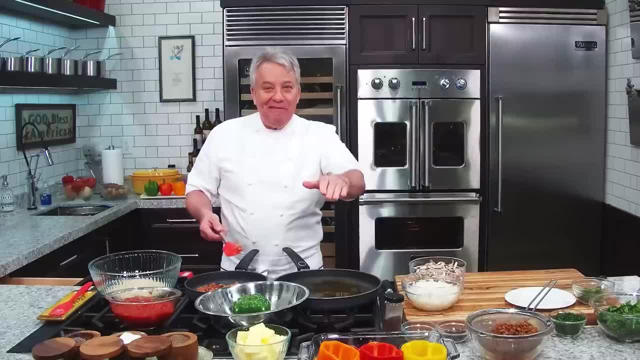 A crook and cronny. You know, like when you have an English muffin, you know the crook and cronny. I don't know what they call it right, But you need that. It's really important. Don't cut it with a knife. 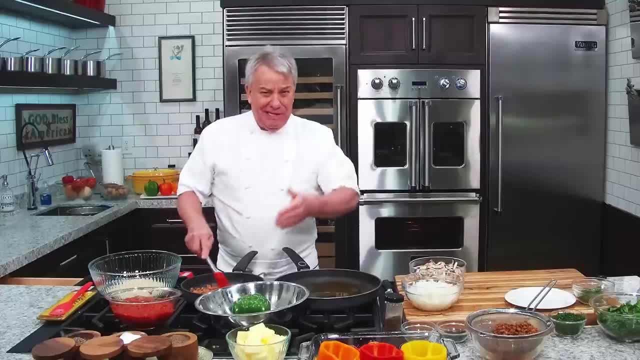 Sometimes you go to a restaurant, big Italian restaurant, and they put in a food processor. Mamma mia, don't ever do that. You're like baby food. I'm telling you. you don't want that, You want to create that. 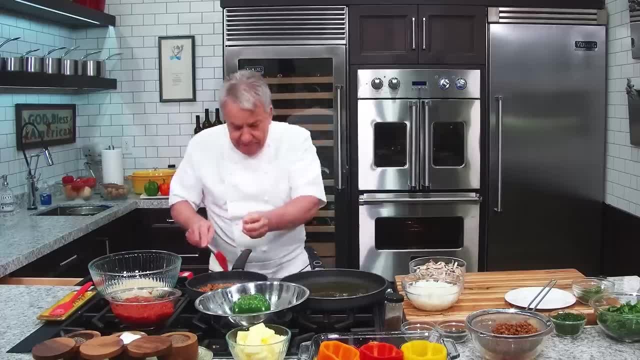 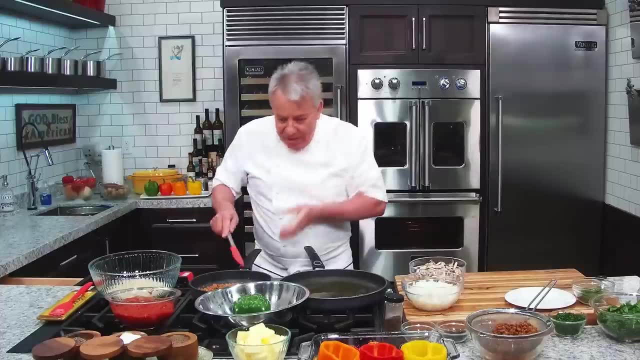 I don't know what you call it. You know what I'm talking about. The round and all that stuff is really, really important. Remember, texture is a conductor of flavor. So if I give you baby food instead of giving you that big difference, all right. 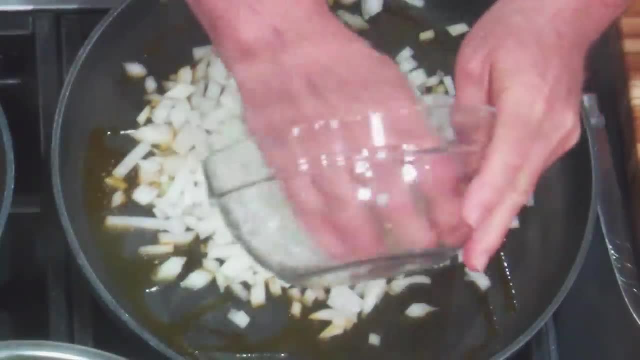 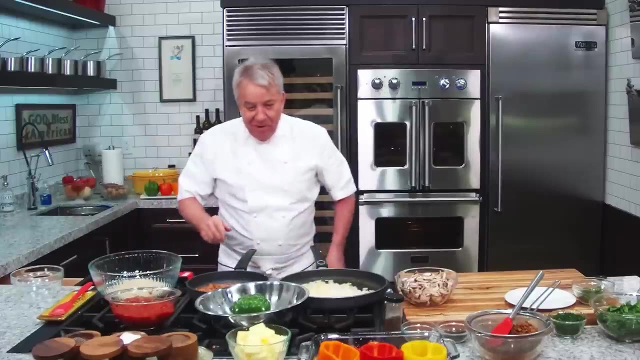 Okay, I'm done with this. Let me put some onion in there. And I got one large onion, One large onion. That thing was big. let me tell you, This is one big onion. You remember Justin Wilson? I love this guy. 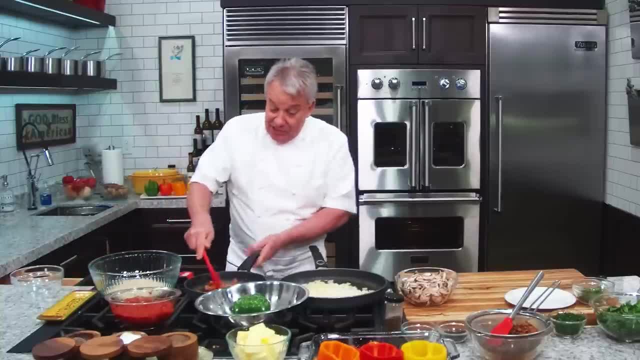 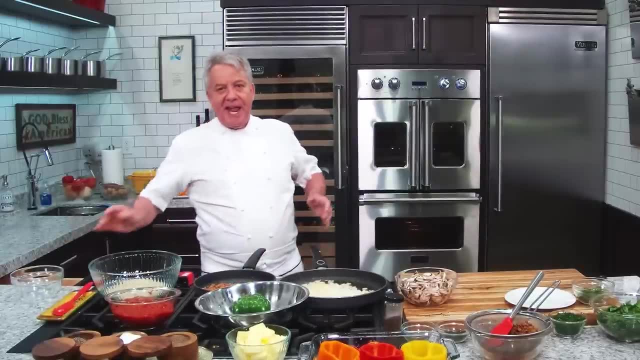 I grew up watching Justin Wilson. I mean that's aging, But that's okay. You know what I got? no issues with my age. A lot of people were watching Justin Wilson. I guarantee that. Remember he had the suspenders. 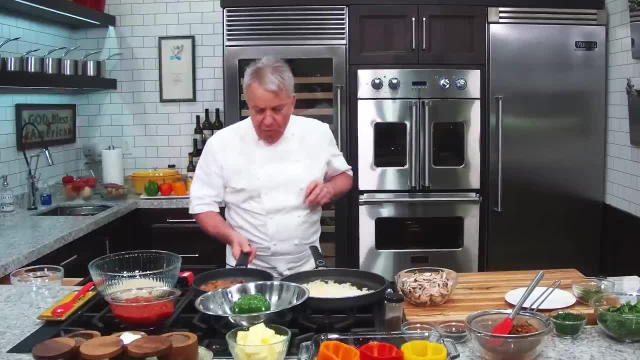 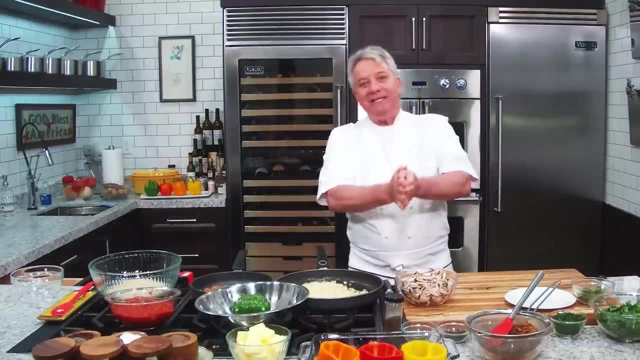 I guarantee them onion are really good. Good onion, He was good boy. So anyway, I love Justin Wilson. May he rest in peace. Okay, so, mushroom, we're going to put them in a minute. Let's get the peppers ready, friends. 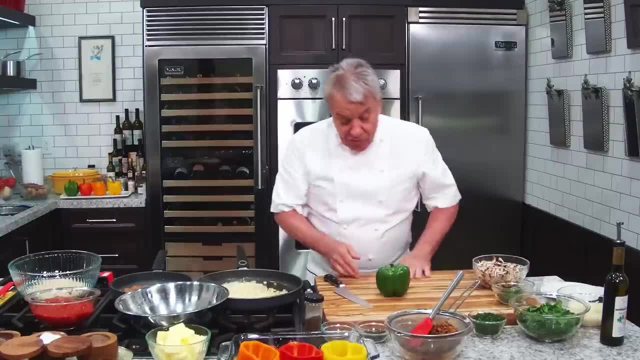 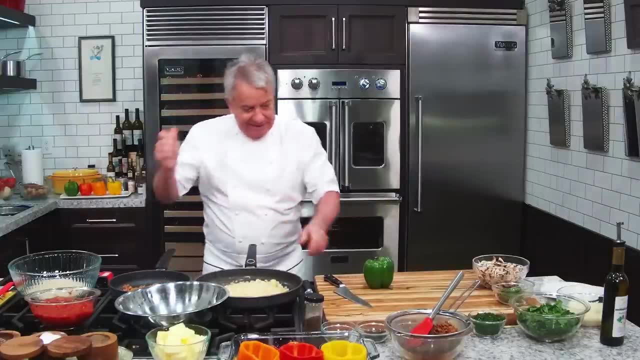 Look, I got the peppers right there. Try them. Mamma mia, Try to buy them. Imagine the people not here for the first time on our channel. They are already gone to tic-tac-tock because the video is too long for them. 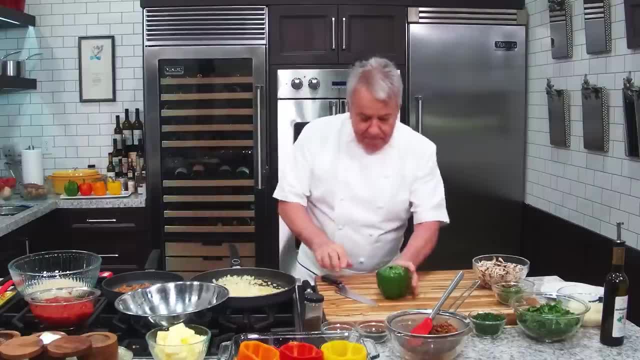 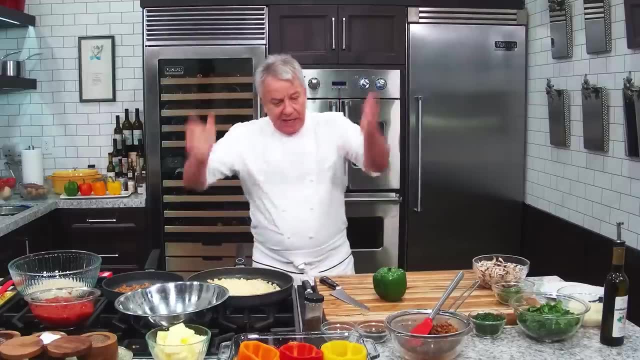 God bless them. So look guys, The peppers you want to try to find them when they're straight. It's not easy. let me tell you, I was at the grocery store today. It took me like an hour to find peppers that are straight. 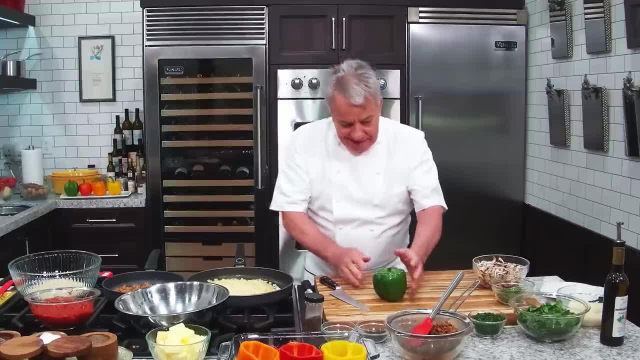 Everything is crooked These days. I don't know what. it is. All right, so try to find them when they're straight. This lady was behind me and she goes. you know they're all the same. I said: well, I like them straight if you don't mind. 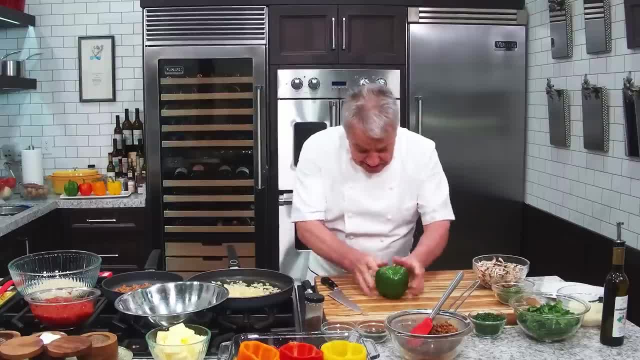 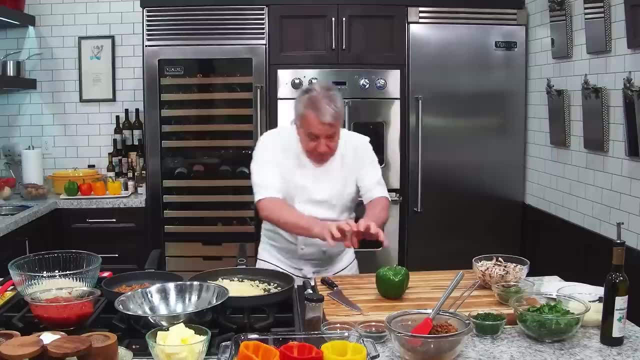 Oh boy, She didn't like that too much. So look this guy's straight. but I got a trick I'm going to show you in case you can't find them straight. You know, I had them in a shopping cart and I'm putting the peppers and I'm looking at all them and all people are looking at me. 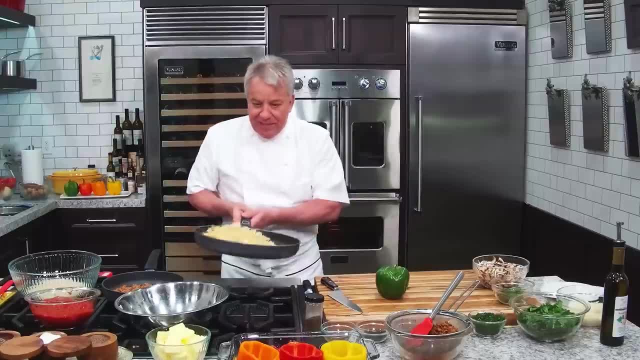 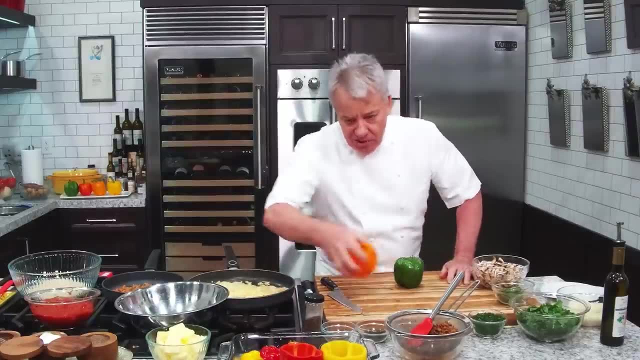 These guys are nuts. He's looking at these peppers. I wanted them the same size and I wanted them to be straight. Guess what? These guys are crooked. See that. Look at this. That's okay, I'll show you. 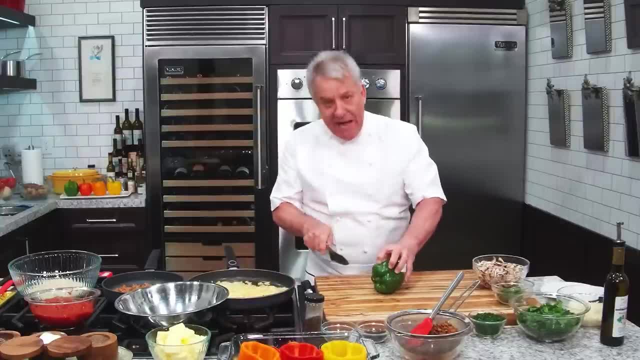 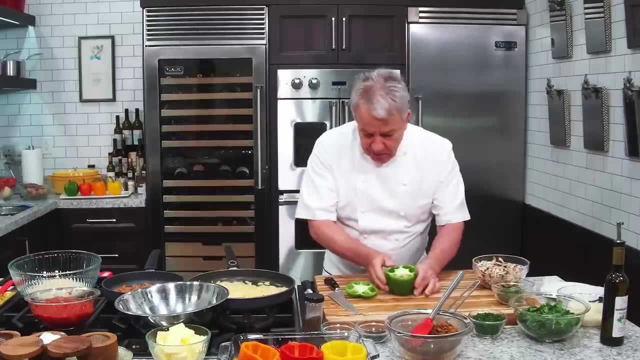 We'll fix them. All right, let's cut the thing in half. Not in half. We just want to cut away. It starts to go like this: We want to cut it. Okay Now, what do we do with this? 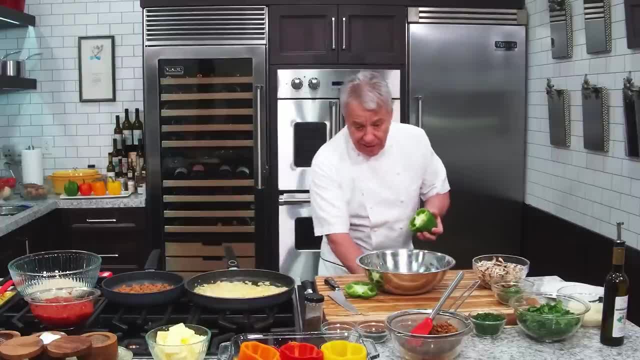 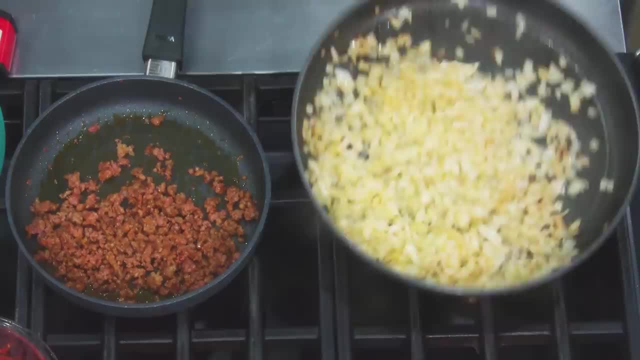 Oh, let's get a bowl and we should take a little knife. Let's make sure we're doing good over here. okay, We're doing good over here. We're doing good over here. I want to get the onion caramelization first. 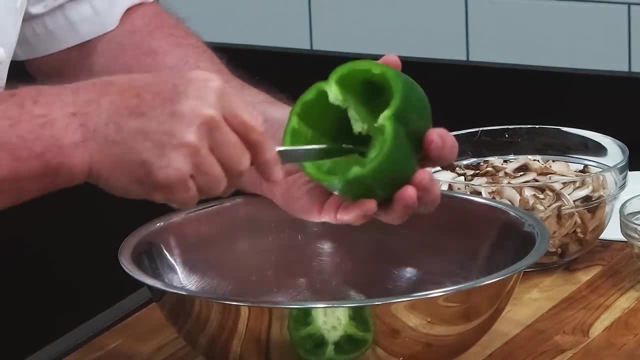 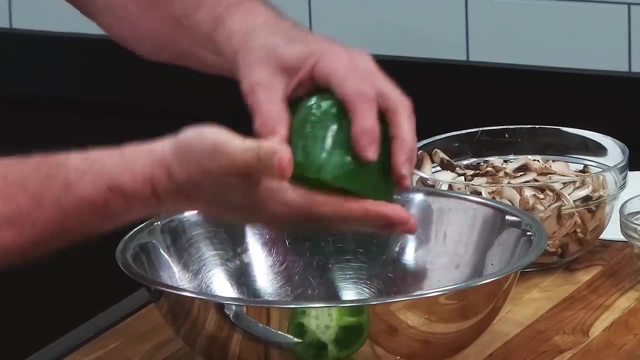 Remember the onion, It's always number first. okay, Don't forget that. All right, You take a little bit of light right there And you may just take a spoon if you're, Or you go like this: See, They come right out. 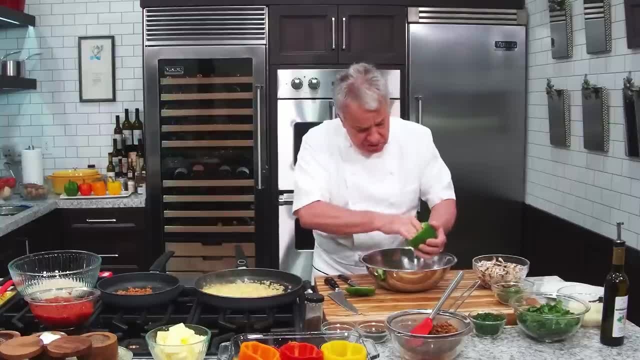 Look at that. Not one single. Oh, my bowl is hot. It must have been on the stove, All right. So look, We got this guy, We're done. What are we doing now? Oh, we do one more thing with it. 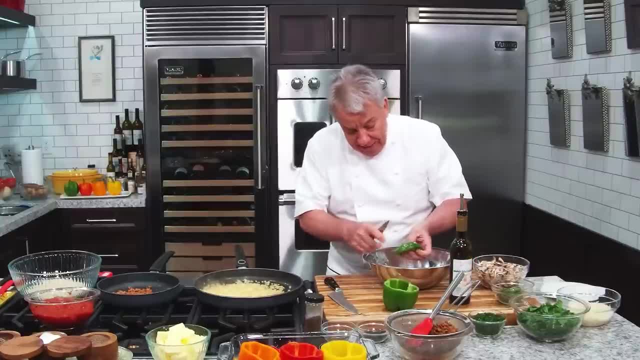 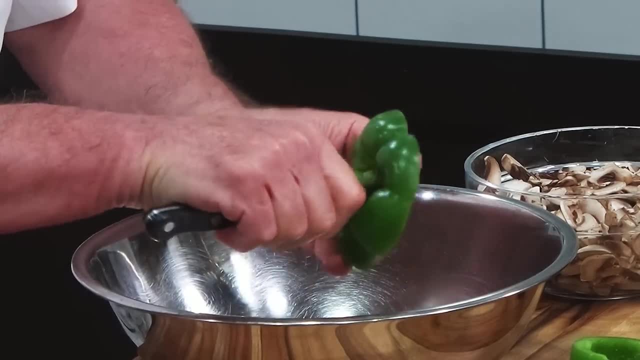 First, we want to remove this stem. Be careful, See. It's not coming out. So be careful. Take the paring knife And be gentle. now You want to remove this stem, You'll see, You'll see. 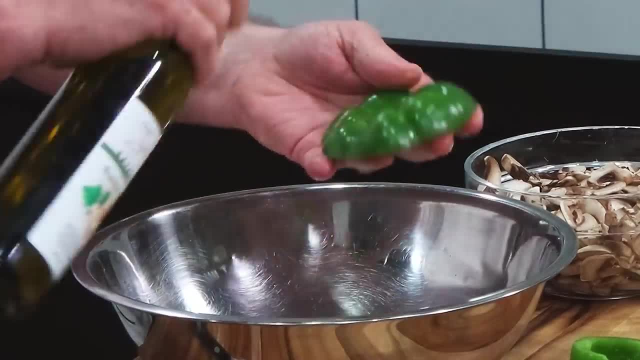 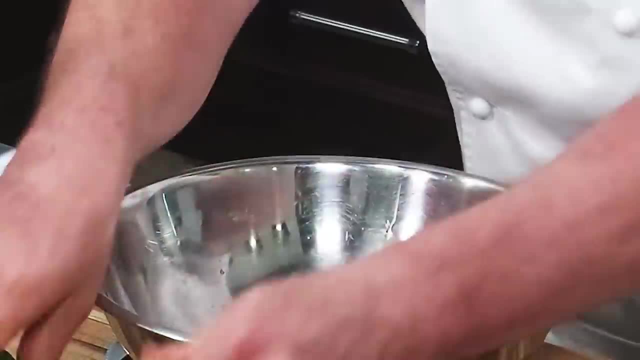 You'll see You're going to like it All right. Then you take a little bit of olive oil. Hey, look at you, Come out. I'm using my garlic olive oil And I rub it all over. A little bit of garlic olive oil. 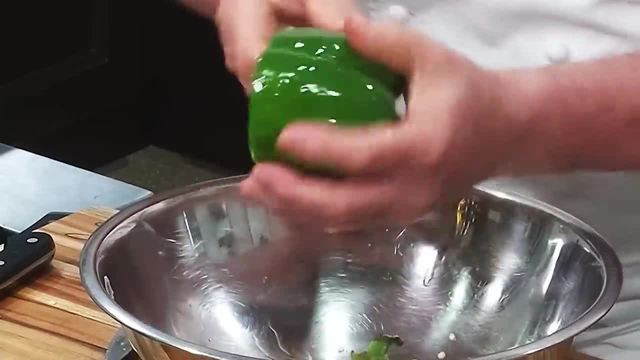 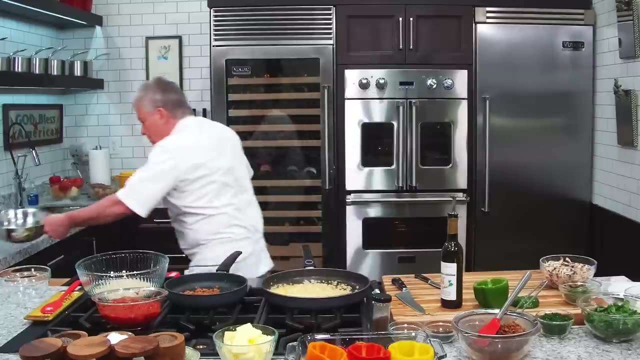 Right, Rub it all over. All right, Rub it inside, Rub it everywhere And be generous. And let me, Let me go wash my hands- Keep an eye on the onion. okay, guys, They can't keep an eye on the onion. 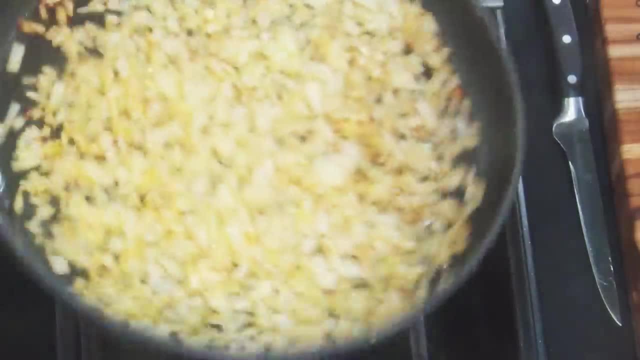 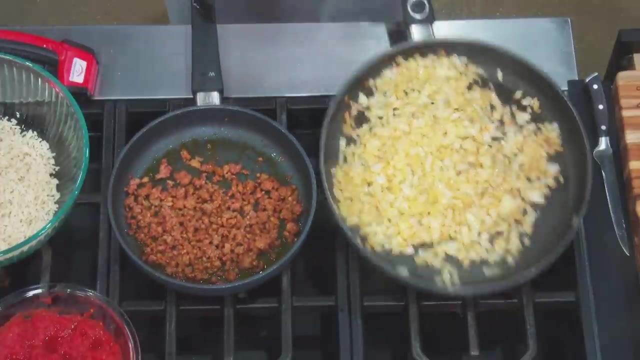 They're on the other side of the camera. Here you go. Look, Oh, mama mia, Almost burned the onion. The sausage is done. friends, Let me turn this off so I can take a breather. Here we go. Mushrooms. 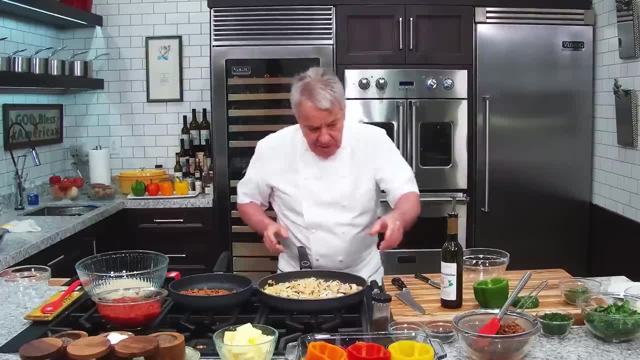 All right For the mushroom. we want to get rid of the water, So I'm going to put a little bit of salt And I'm putting my mushrooms Mushroom salt. I don't know if you've ever used my mushroom salt. 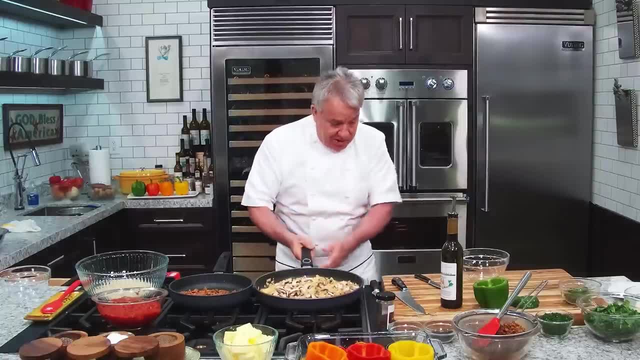 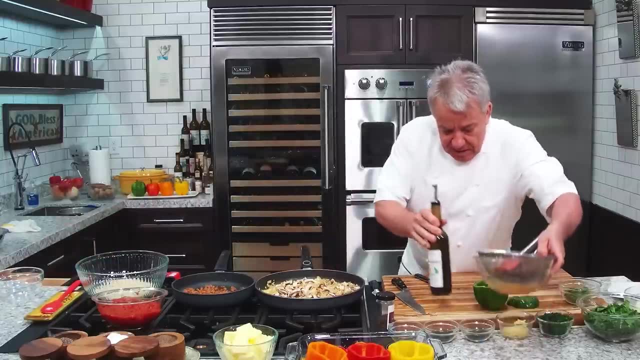 It smells delicious. Dry porcini mushroom. It's delicious. All right, Now what do we do with the sausage friends? What do we do with the sausage? We take the sausage. Let's take the peppers out of there for a minute. 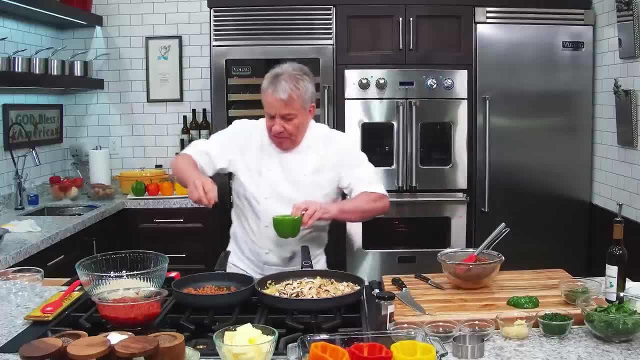 Did I put the salt in there? No, I didn't put the salt. You got to put the salt in there. friends, Take a little bit of salt, Put it right in there, Inside, outside. I already got the other ones. 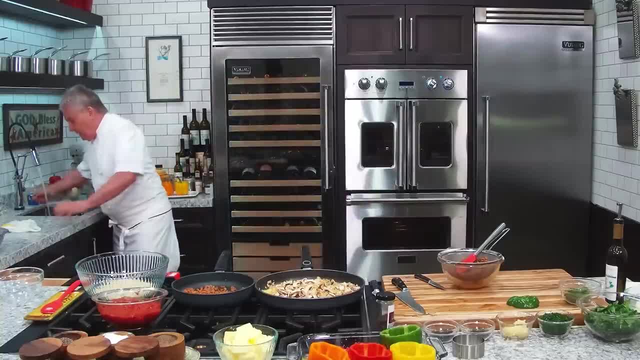 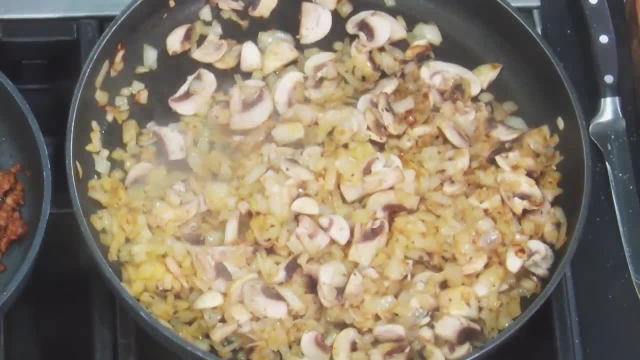 I got to wash my hand again. I should have a sink right there. Right there, Let's make sure we get rid of the water in the mushroom. Everything is in order. right, Take the sausage right there, friends, Put it right there. 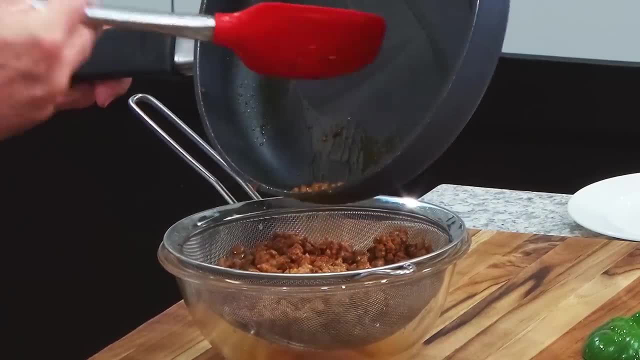 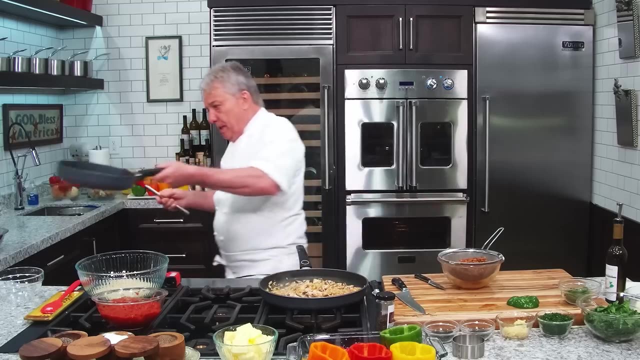 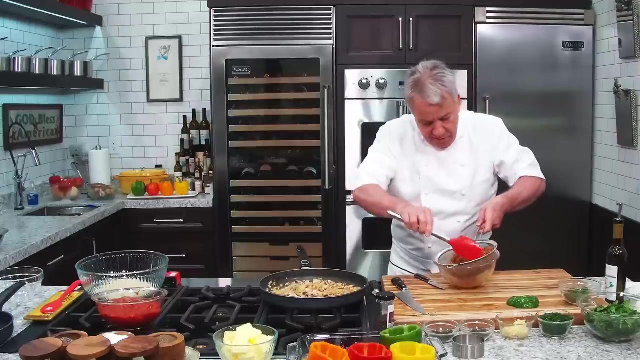 Right there Now. don't leave any of the fat in there. We love that pork fat. We love that pork fat. friends, Take it right there. All right, Mix it up pretty good. See, Look how beautiful that is. 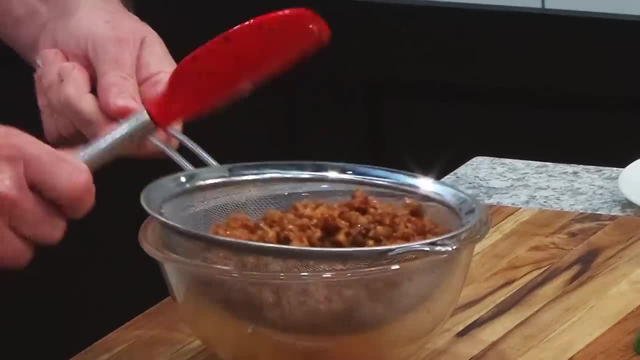 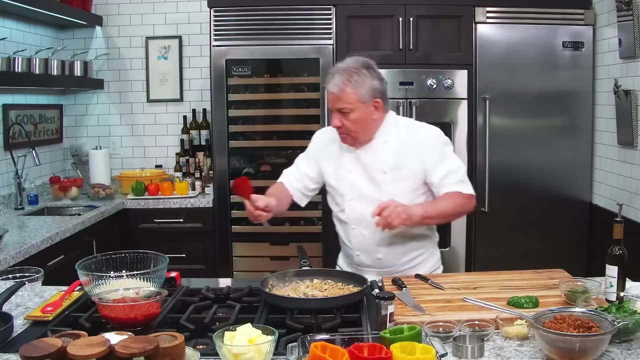 See, See what I'm talking about. right there, folks, Right there The Maya reaction. If there's an extra fat, there's not an extra, All right, We're done with the sausage. Let me not put everything in the middle. 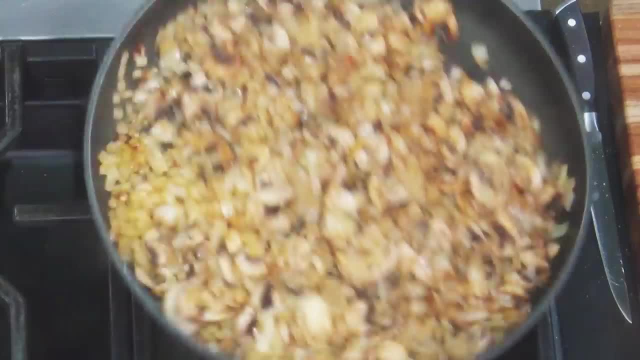 You know what? I'm going to put my spatula here, because I'll use it in a minute. What else do we put in here? It's going to be the stuffing. We're going to put some rice. I got about two or three cups of rice cooked. 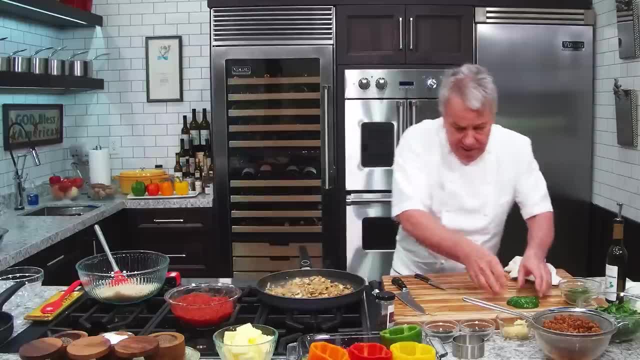 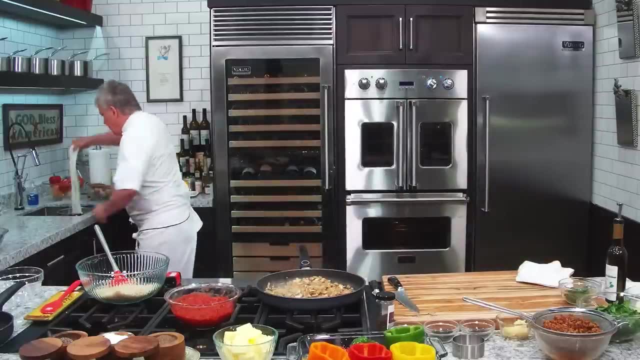 I got some lavallee tomatoes. They're wonderful, Lavallee tomatoes. Let me just clean up my cutting board And then I'm going to put the seasoning in there. friends, There's a lot of stuff to prepare in advance for this. 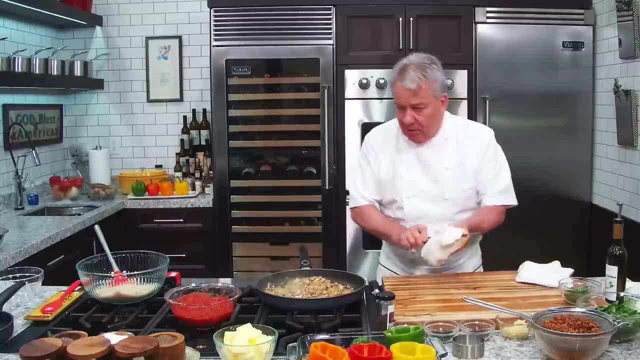 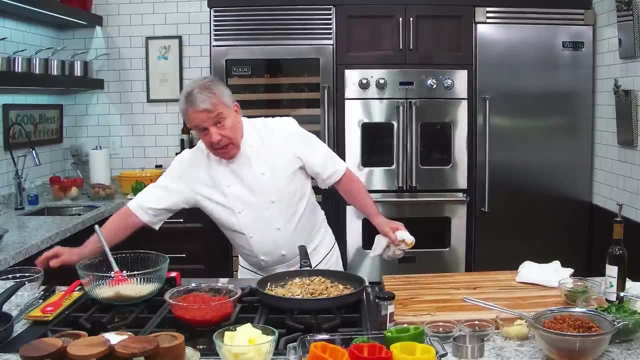 So you know you can download the recipe. We have a lot of people that ask all the time: where is the recipe? Friends, for those of you that are not familiar with YouTube, underneath the recipe there's a link. There's a description. 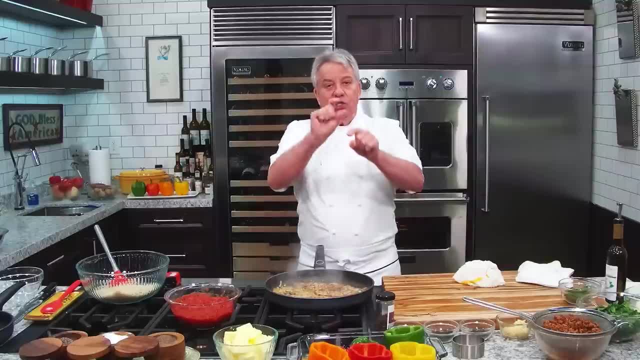 And there's a link And in the link, at the end of the link, it says: show more. You click on that and you have a link to the free recipe. You can go and get the free recipe. All right. 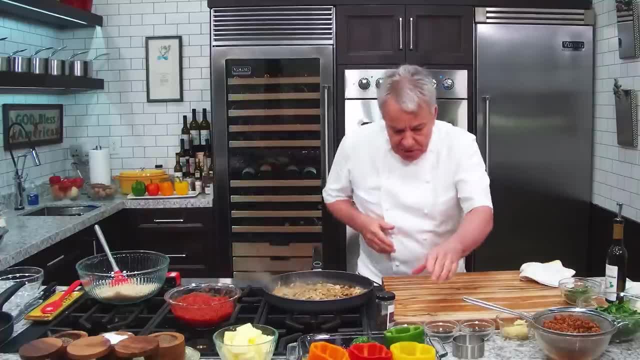 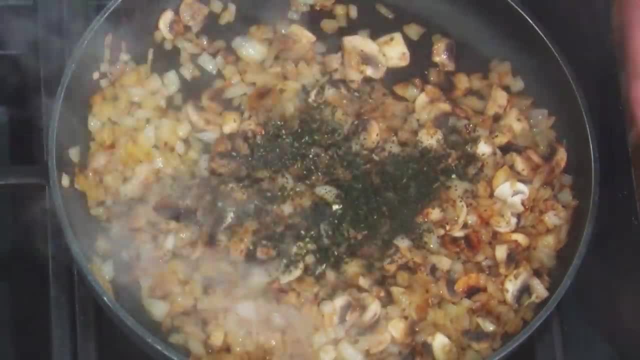 So what else do we put in here? We put some. I got fresh herbs, If you have them, great. A little bit of rosemary, A little bit of oregano, A little bit of thyme. Put whatever else makes you happy friends, okay. 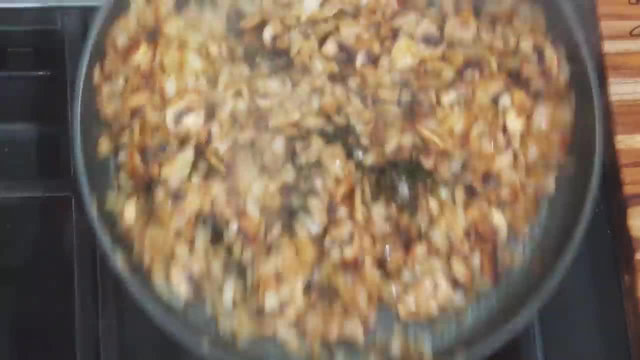 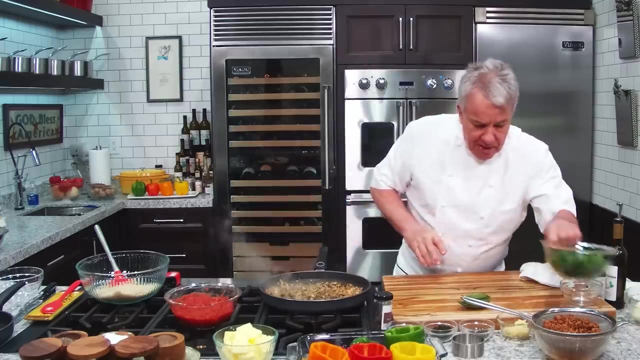 And I'm going to put a little basil in a minute, Mix it all up. Okay, it's looking good. so far, right, Very simple right, No big deal. We're going to put a little spinach, We're going to saute this. 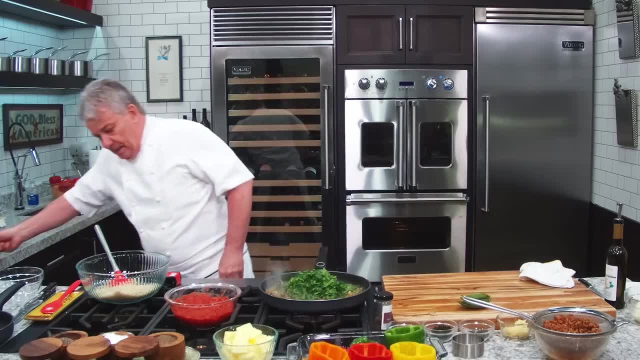 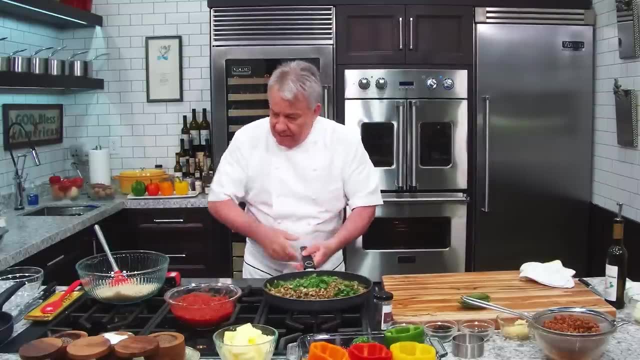 And then we're going to put some tomatoes- Yep, We're going to mix all this up, friends, And then we're going to mix it with the rice, And then we're going to stuff it all. I'm telling you, this is really really simple. 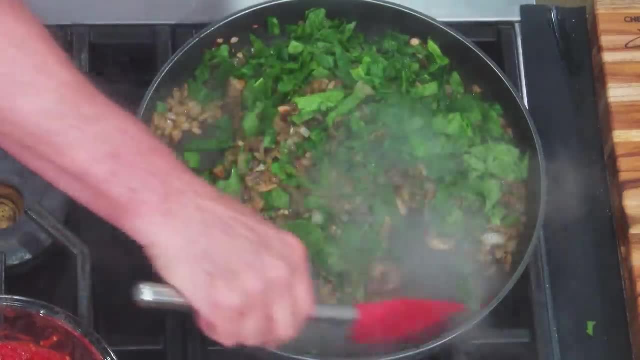 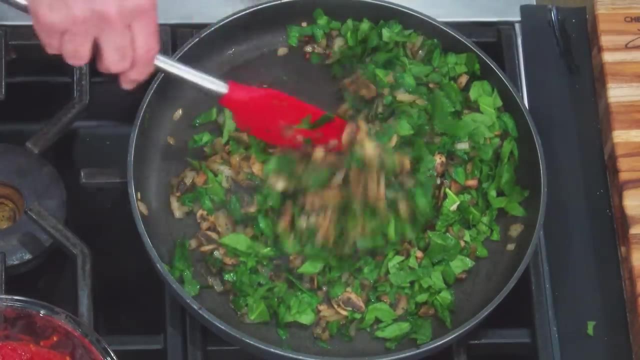 But I'm going to show you We're going to- first, we're going to cook the peppers. I'm going to show you We're going to do a bunch of stuff. This is really delicious. This is so delicious, especially with the sausage. 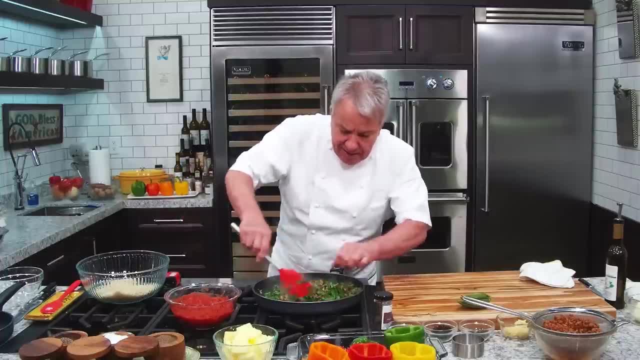 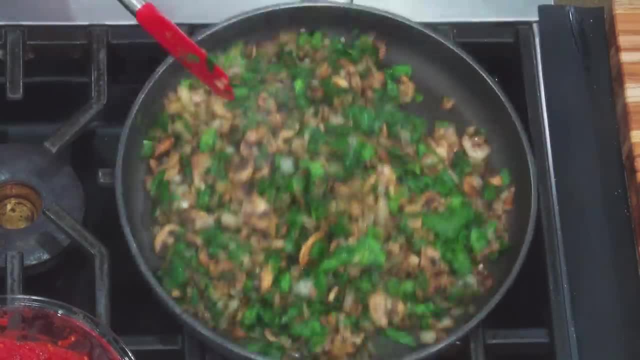 You can make it with ground beef. You're going to make it with ground beef. Make it with 80-20,, 80 lean, 20.. If you can make your own ground beef, it's great, But if you can't, then get to the butcher shop. 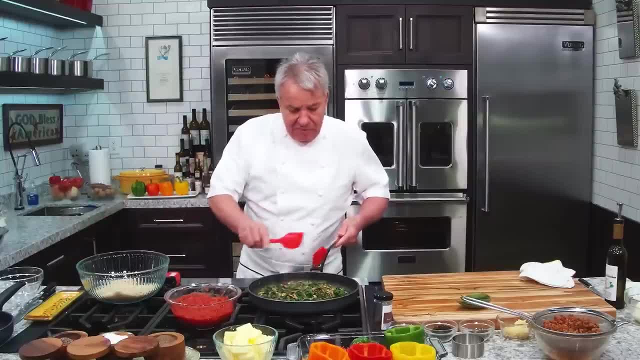 Try to go to the butcher shop Grocery store. they're not so good. They're not so good with the ground beef. I mean some of them do. I shouldn't be picking on grocery store because some grocery store do it themselves. 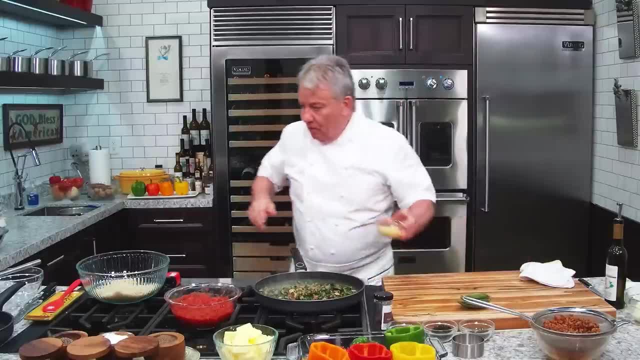 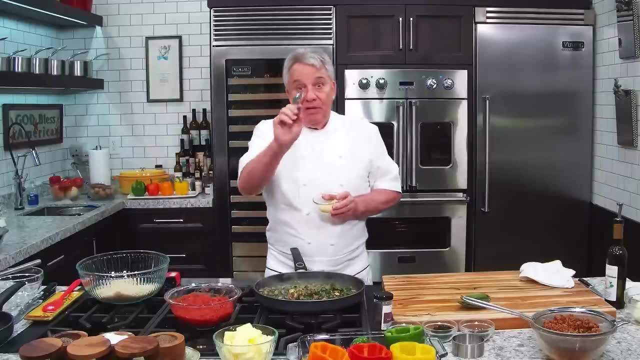 I can smell the herbs. They smell delicious. We're going to put a little garlic in there. friends, Now, when a minute we put the garlic, that means what That means. we're getting ready to put liquid Tomatoes. Okay, remember you don't put the garlic. 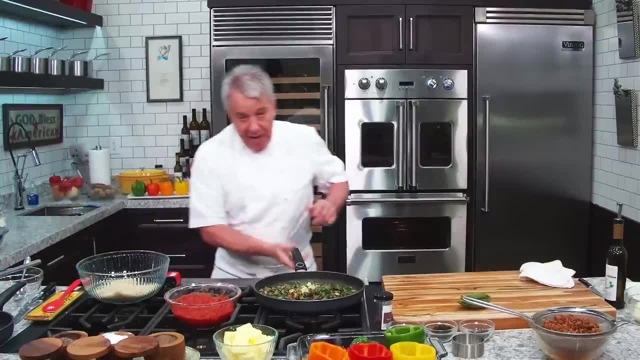 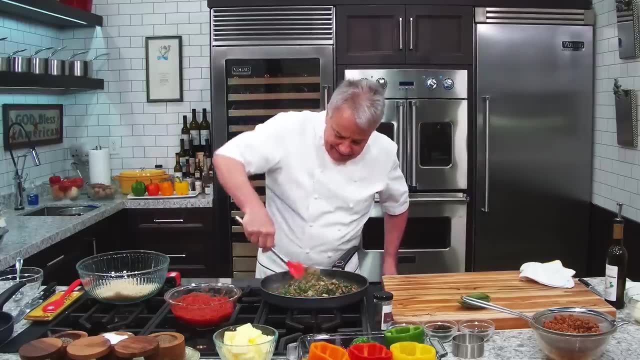 at the beginning of a dish, Otherwise you'll burn it. It becomes bitter Instead of fragrant floral, delicate. it's bitter right. So here we have it. Here we have it. We're smelling it The minute we smell it. 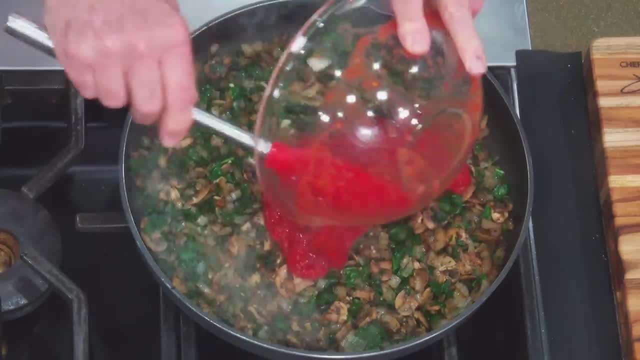 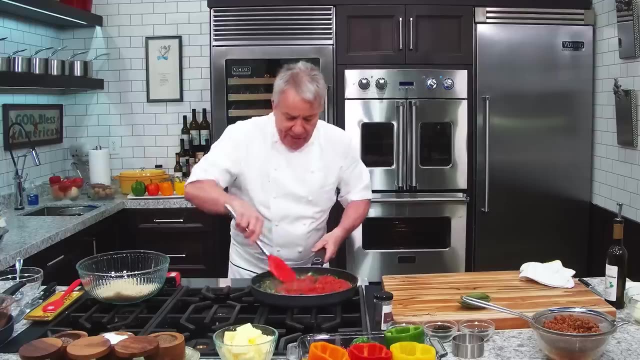 we're now going to put our tomatoes in there. Pretty simple, eh? This is about a can and a half of Lavallee fresh Fresh, no, Not fresh, They were fresh when they put them in the can. Lavallee tomatoes are delicious. 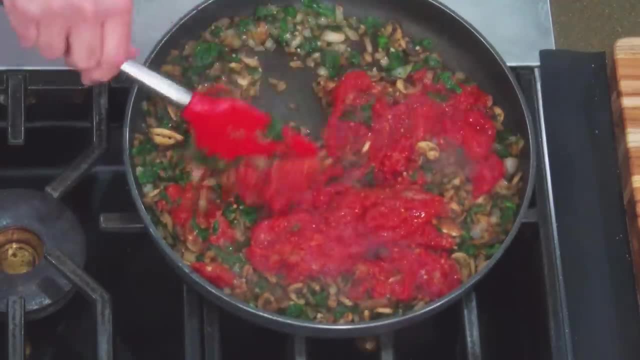 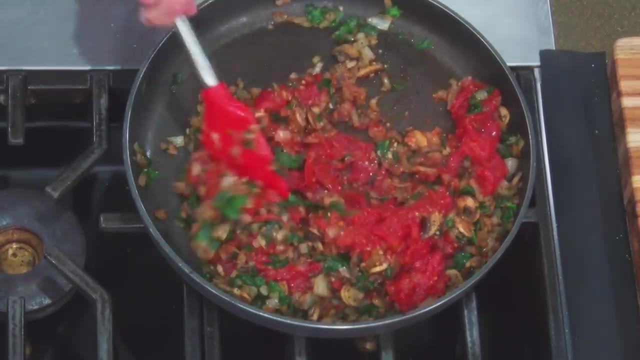 Use a good tomato. Those are peeled tomatoes And they're delicious, my friends, I promise you. It's all about the tomato you're using. You make a good tomato sauce. you need a good tomato. That's all it is is tomatoes. 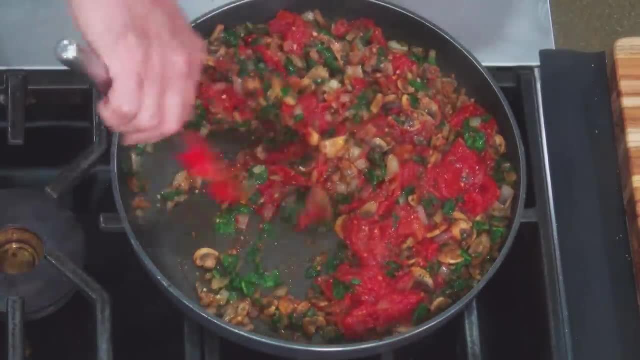 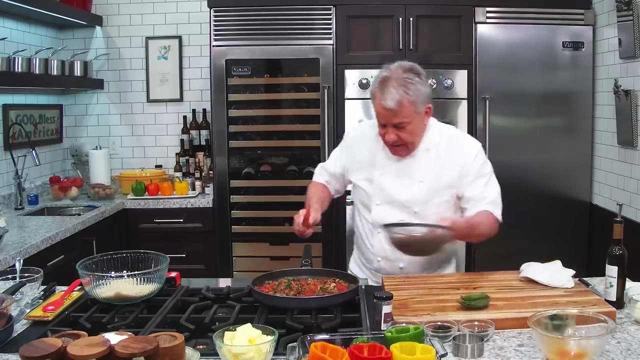 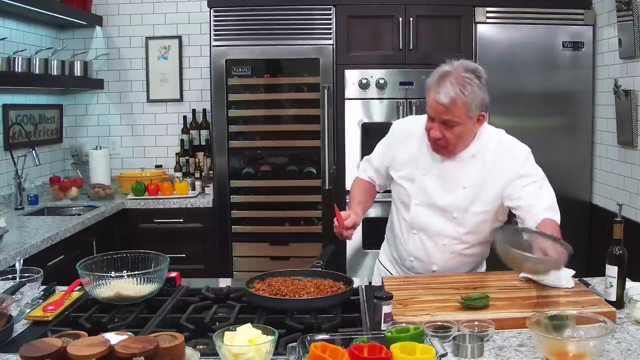 Right, What do you think We're looking good so far? Well, let me tell you We're going to mix the sausage with this Right Right now. Yeah, Yeah, If there is a little extra fat in here, we're going to use it because we love it. 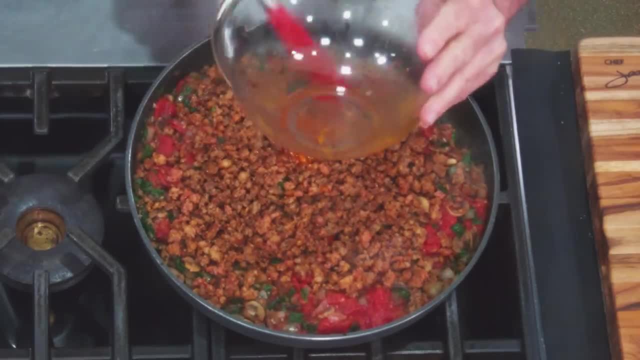 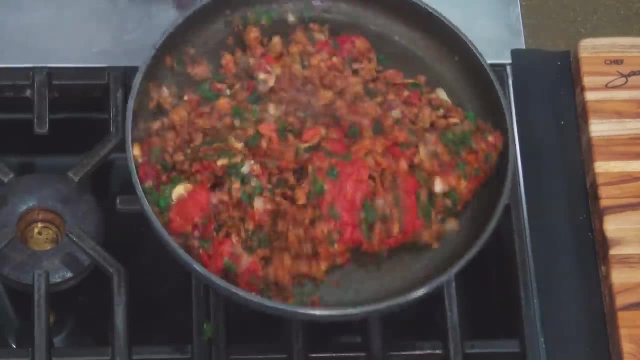 It's delicious From the sausage. There you go. Just a little bit So we don't waste none. I don't like to waste anything, my friends, And we're going to mix all this with the rice And then we're going to stuff the pepper. 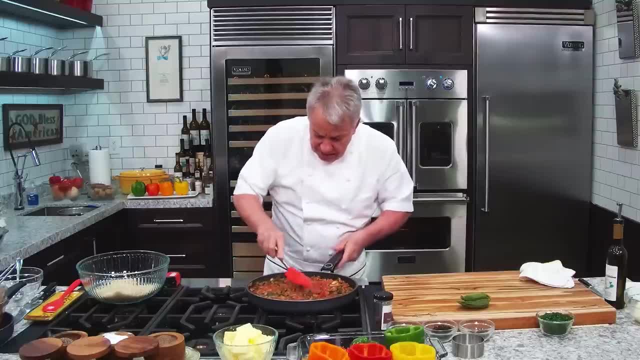 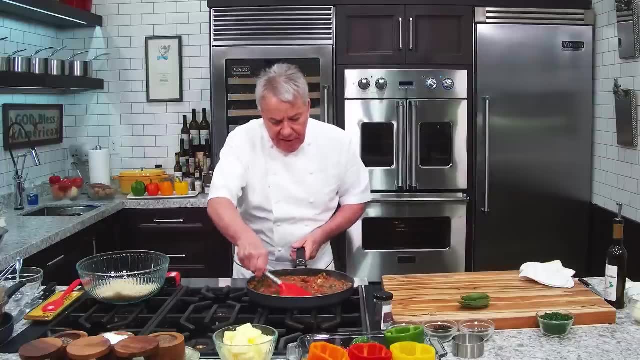 All right. So we're going to cook this slowly for a good 20 minutes, my friends, 15,, 20 minutes- Very, very slowly, because we're going to finish cooking the whole thing. We're going to finish cooking the whole thing. 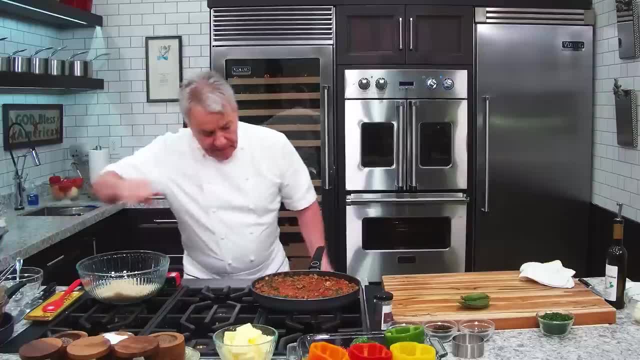 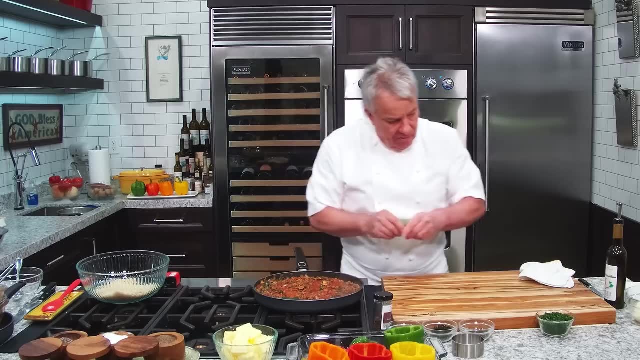 We're going to finish cooking the whole thing in the peppers, But what do we do with the pepper now? Just before we put the pepper, we will put the basil in there. I don't want to overcook the basil, So the peppers. 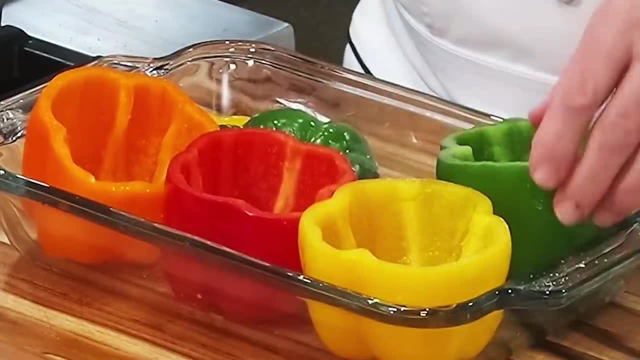 What we're going to do with the peppers. we got them with the oil in there. We want to save those. You see You're going to love what I will do with this. This is very cool. So remember, we save them without the stem. 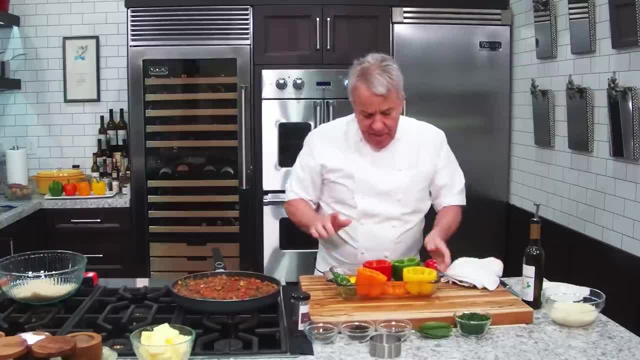 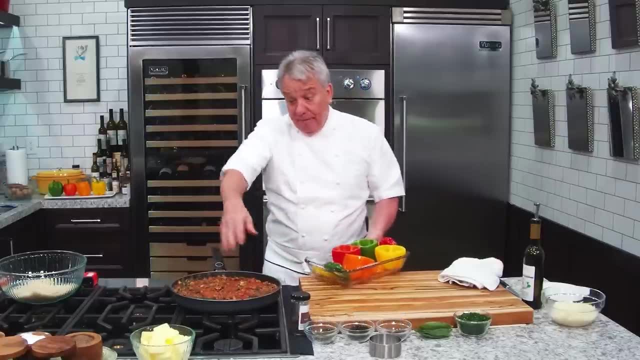 Okay, Doesn't matter how you do it, Right in there, They're going to go in the oven. The oven is 350.. 375 depends on your oven. For about 20 minutes we're going to parkook them before we stuff them. 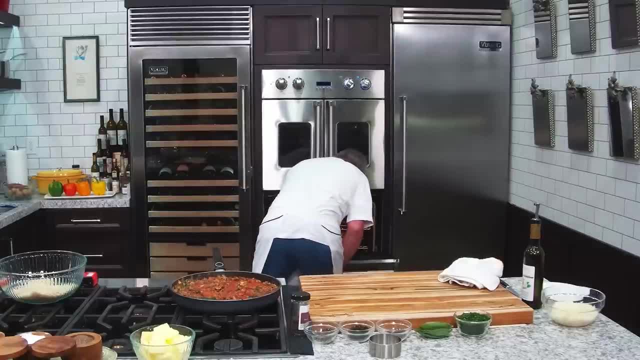 All right, So we're going to put them right there in the oven. We're going to look at the clock. We're going to put ourself a timer for 20 minutes to make sure we don't forget. We got the rice right there. 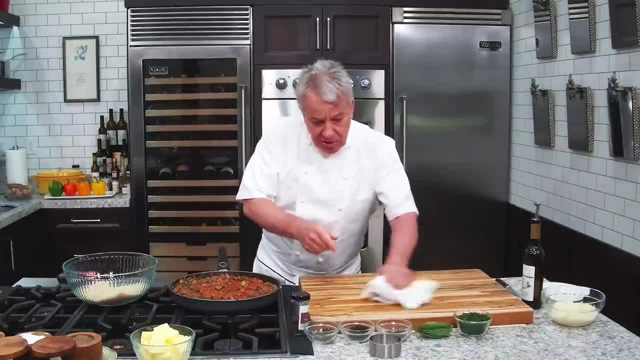 We're going to let all this cook and we're going to mix it all up. The last thing we're going to put in is put in a little basil. We're not just seasoning if we need to. So we'll be back in about 20 minutes. 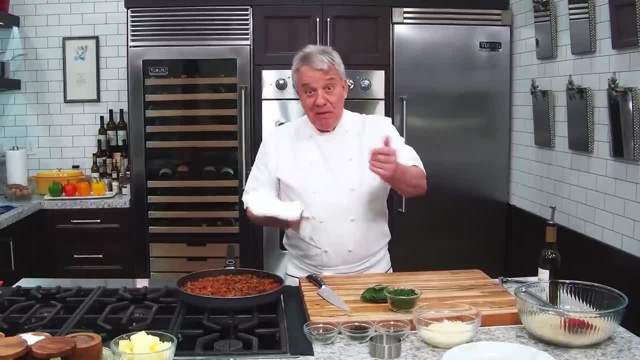 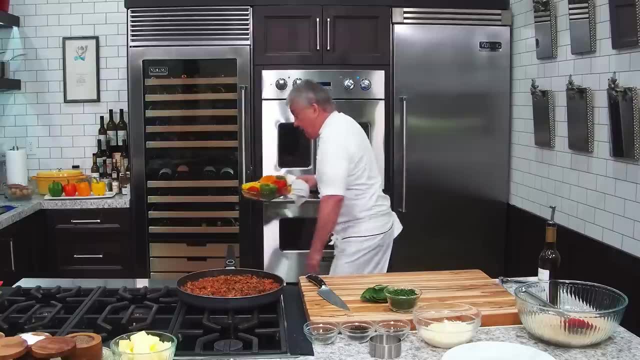 And for you it'll be just a flash. Okay, friends, It's been about 20 minutes, The peppers are starting to cook. I mean, they're not cook, cook, cook, but they got a good head start. So what I'm going to do now, friends, 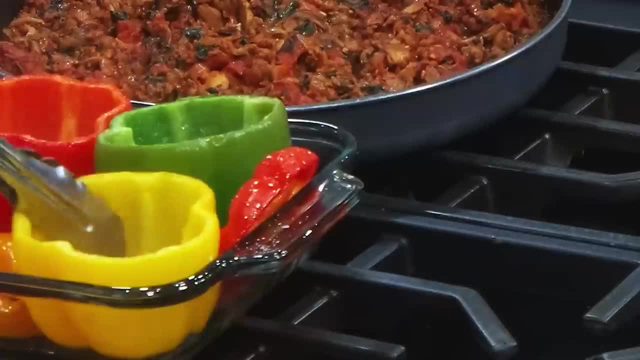 I'm going to remove the water out of them. You see, They have released some water and the water we don't want to throw it away. It's got a little bit of olive oil in it. We're going to take it and we're going to use it in the bottom of the pan. 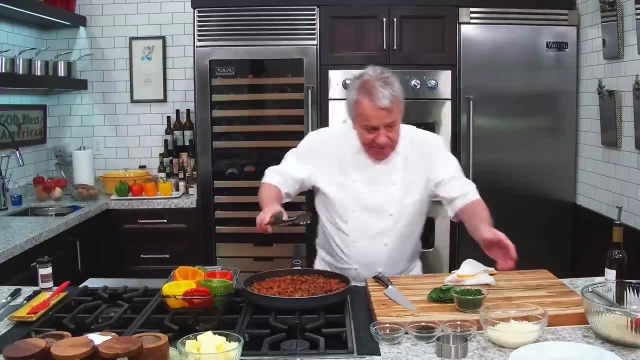 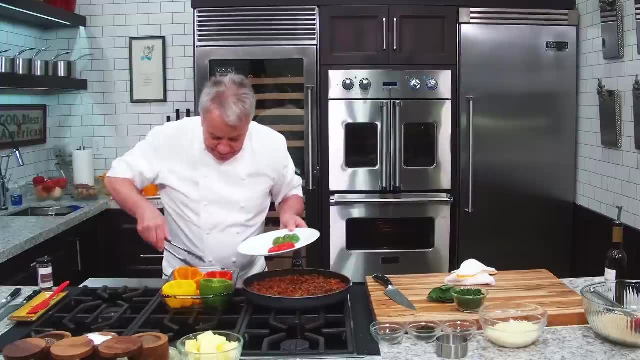 You see, Take it in the bottom of the pan And the tops, the tops. they're not completely cooked, but we're going to, We're going to be good with it because you watch what we're going to use them for. 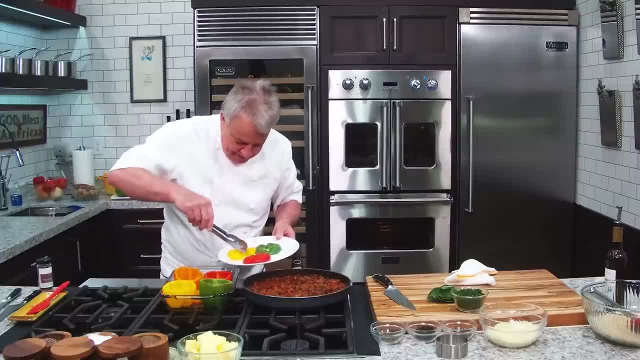 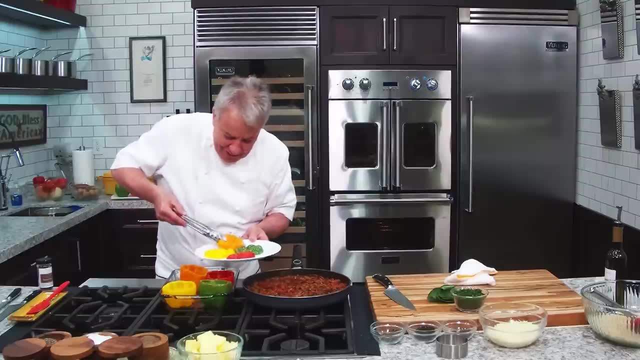 Oh, mamma mia Broke the yellow. Well, don't break the yellow, You see, You see. You see what I'm going to do with them. okay, We're going to leave them here. We use them later, okay. 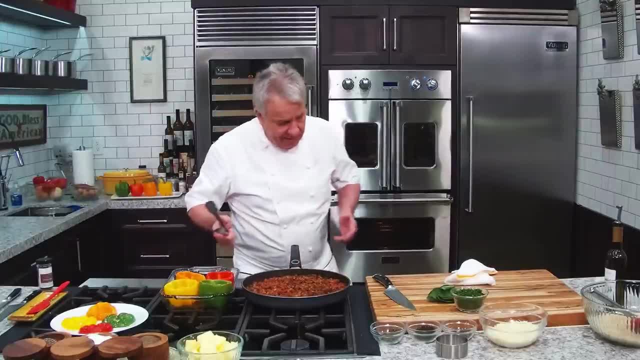 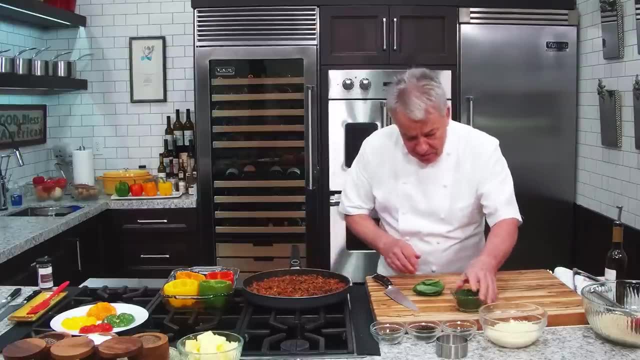 Now, it would have been nice if I had two more, but I don't know. I was uncalculating correctly. That's okay, We're good. Now we're going to put in this. Let me turn this off, I don't need to cook it anymore. 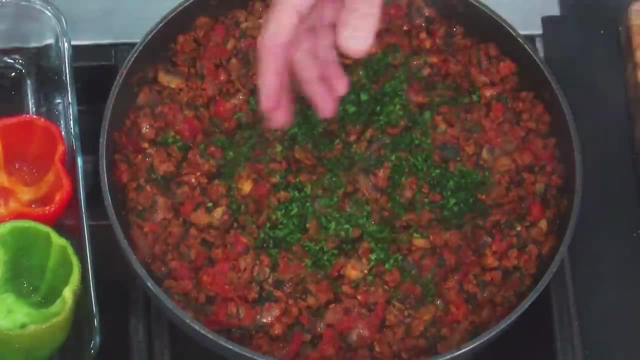 I'm going to put some chopped parsley. I didn't need it to cook, right, So I'm putting it here And I'm going to put a bit of basil chiffonade. okay, And this I like to always cut at the last minute. 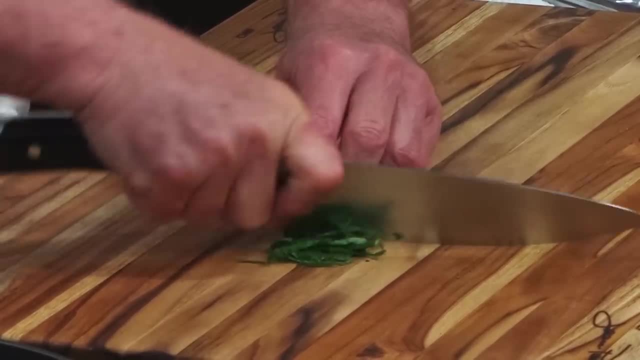 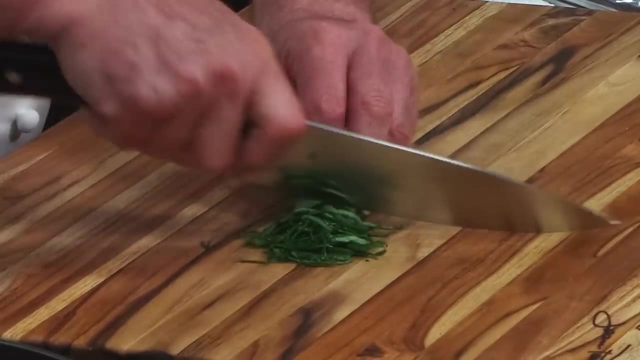 And for those of you that have been following the video, you know exactly what we're doing. We're just cutting the basil in very, very, very small little strips, And this is where you roll it very tight and then you take your knife. 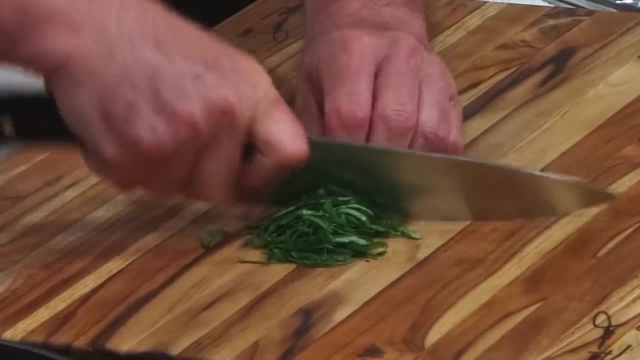 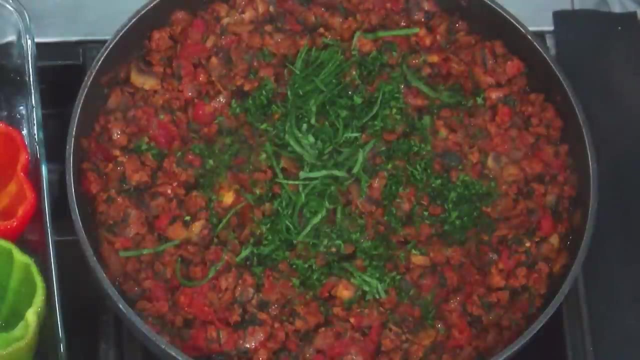 and you give it a very, very, very thin chiffonade, Chiffonade. See, Yeah, chiffonade, That's it All right, I got too many here. Let me put it here. There you go. 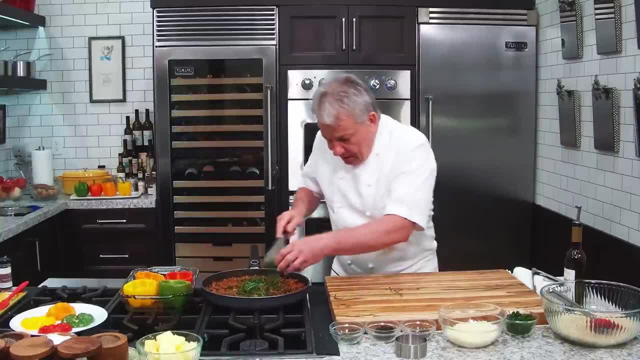 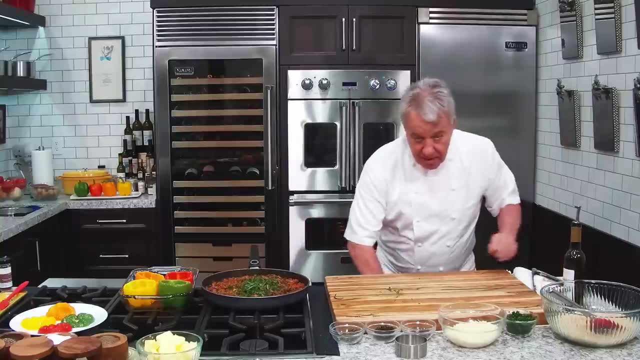 I don't need it. All right, The minute you start cutting this. you don't want to put too much, but you certainly want to put enough. Okay, Don't clean your board with a knife, Otherwise the knife police are going to come and get you. 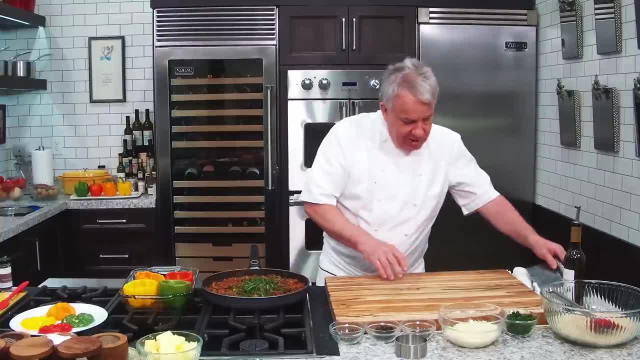 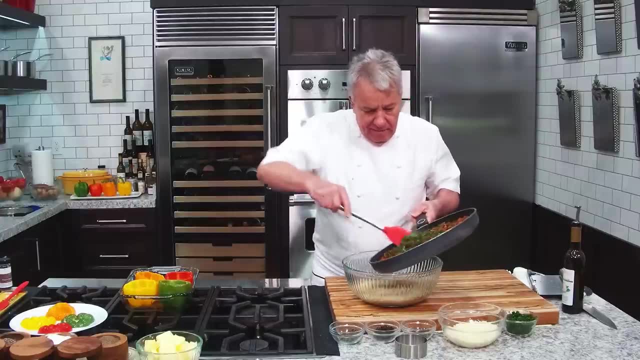 The cutting board right, We're going to mix all this up. And then, friends, we're going to put all this right there, Mix it all up. It's going to get all mixed up in there. We're going to put it with the rice. 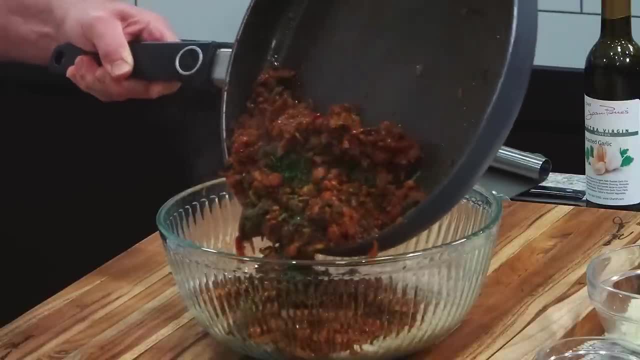 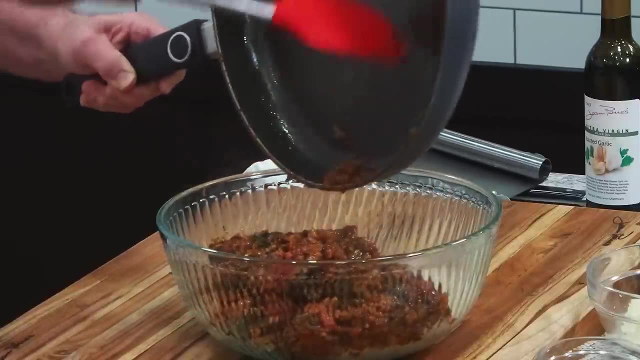 Now, a lot of people put way too much rice for this. I like a little bit of rice, but not too much, eh. So rice is good, Makes it more, gives it more body, Makes it a little more filling also. 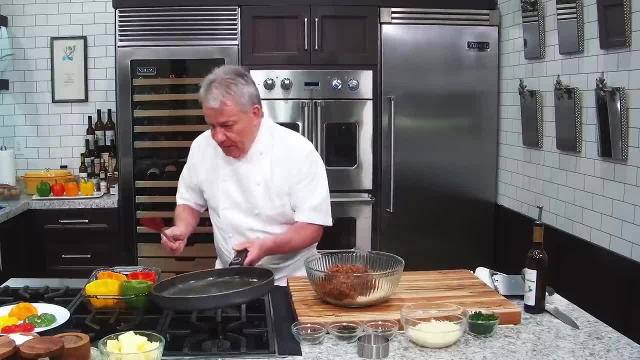 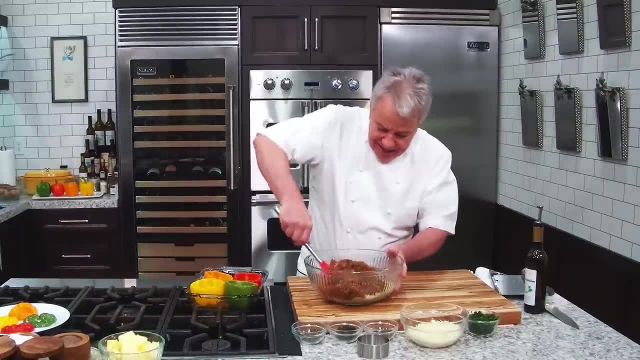 It's really nice, And so we're going to put this over here. We don't need it. Whoo, It's hot, Don't touch it. And then we're going to mix all this up And then we're going to fill the peppers. 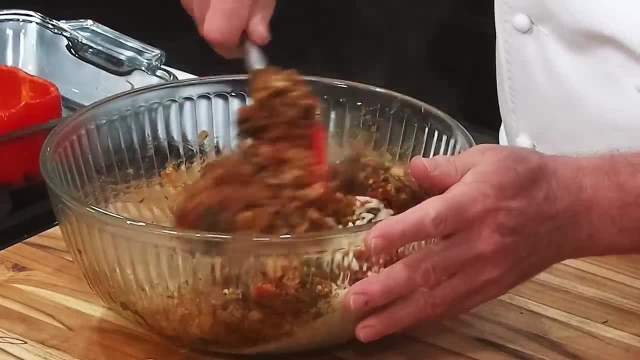 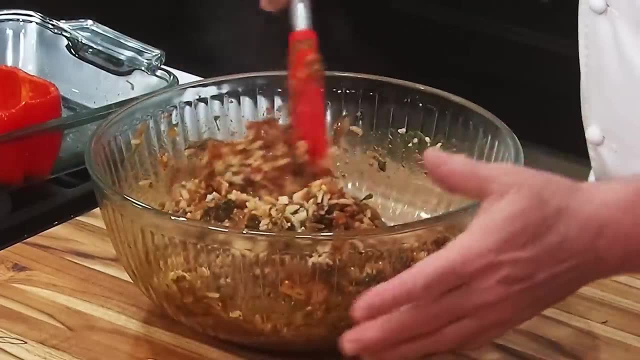 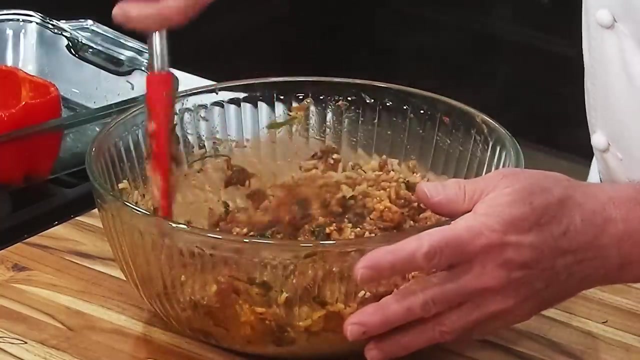 Right, And then we're going to cook them. friends, Again, another 30 minutes, Right, 30 minutes, Maybe 25 minutes? That's a good 25 minutes, Right, We're going to cook them And then we're going to take them out. 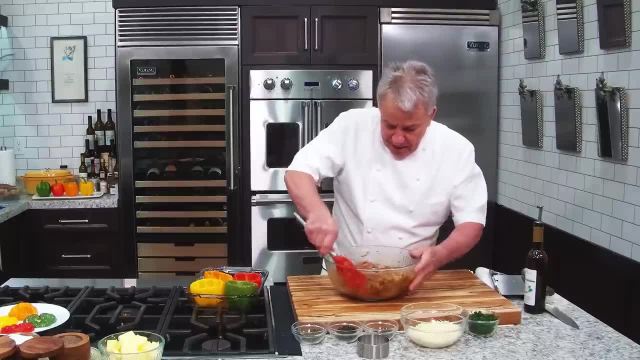 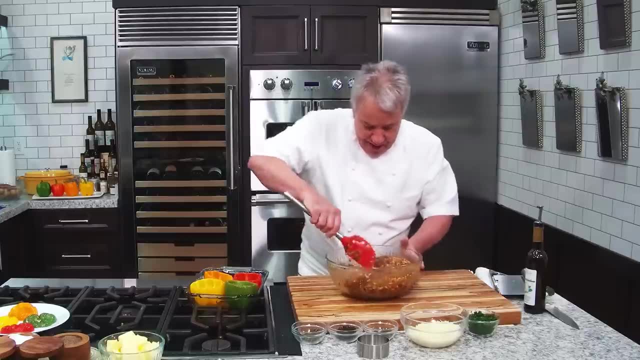 and we're going to put the cheese for the last 10 minutes. We don't want to put the cheese at the beginning because if we put the cheese at the beginning, the cheese will be golden brown and the peppers are not going to be cooked. 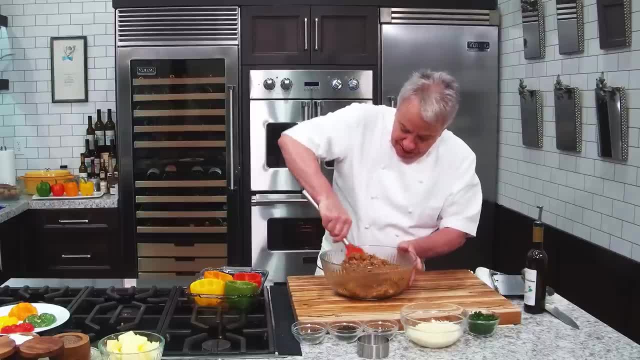 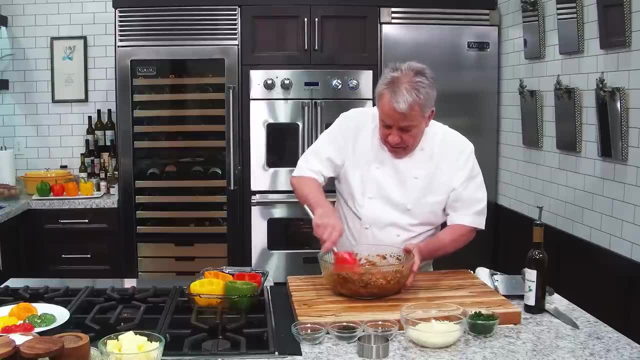 So it's really important, friends, And we do this in three steps, in a way right One: first we cook the pepper a little bit Right And then we finish cooking the stuffing in the pepper. That will finish to cook the peppers. 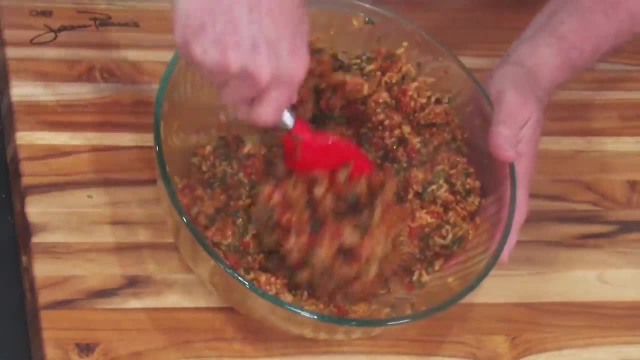 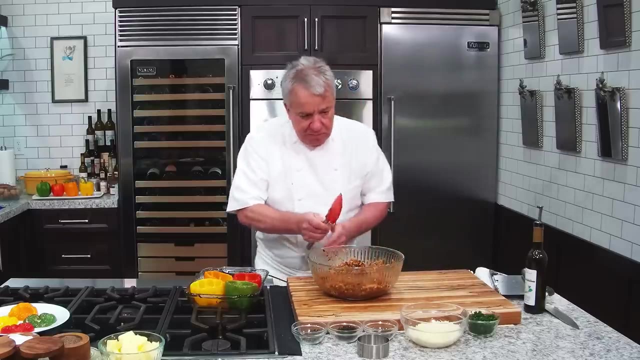 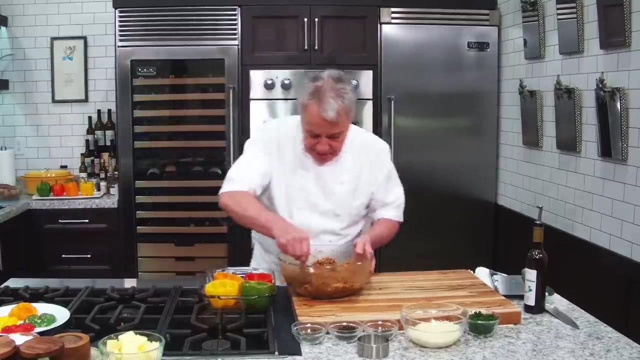 Right. And then at this point I mean: this is delicious. let me tell you- And we take a spoon here, friends, We make a lot of mess right there. You come back over here And we're going to stuff this as best as we can. 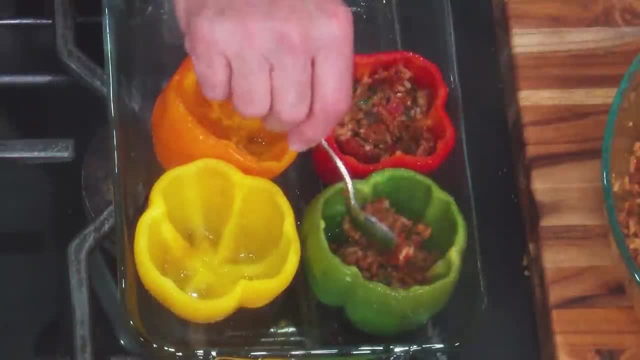 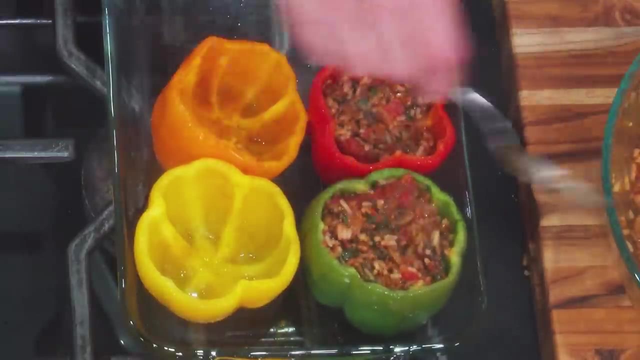 And we're going to give it, we're going to be generous. I always have too much of this, But let me tell you, forget about stuffing the pepper. eh, This right there, It will be amazing just by itself, Okay. 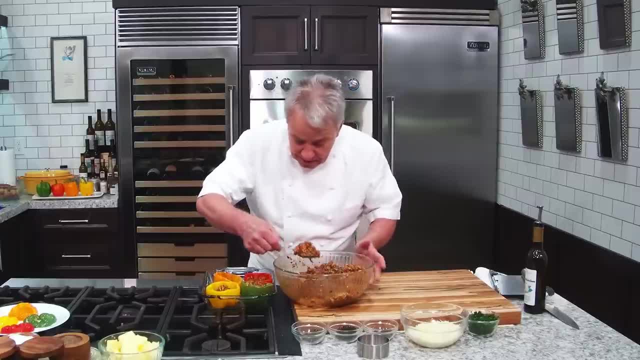 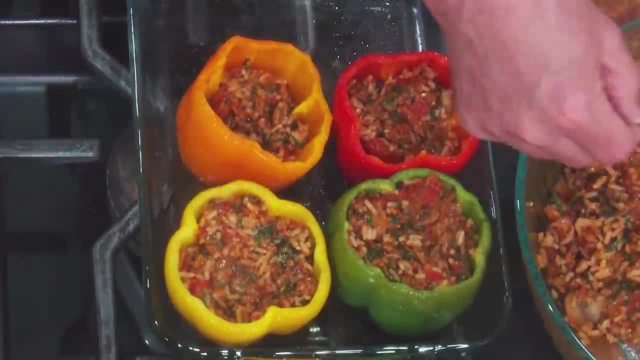 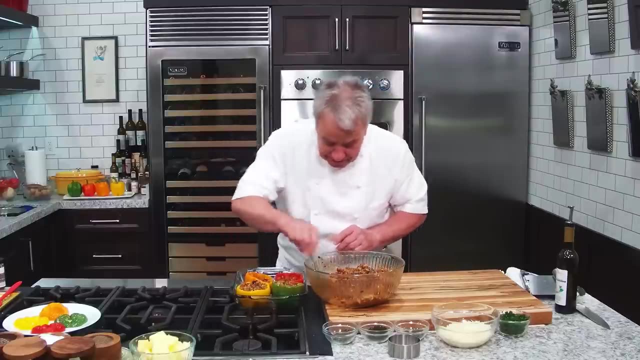 It really is going to be amazing just by itself, Just like this. It will be absolutely amazing. This inside a soft taco, inside a- I forgot what you call those things like a crepe Tortillas. That will be delicious. 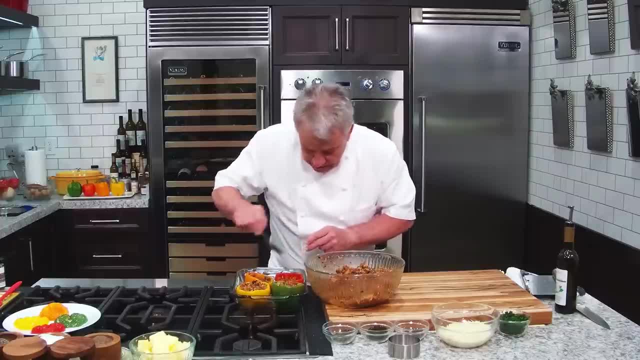 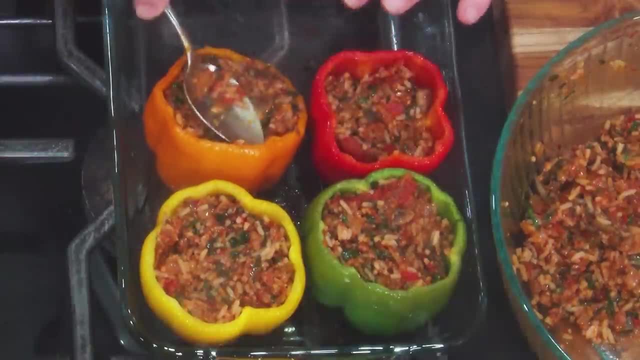 I mean, you can do so many cool things with this. This is absolutely delicious. I can just eat it like this. Now, be very, very, very generous here. Pop it in Really. push it in my friends, Okay. 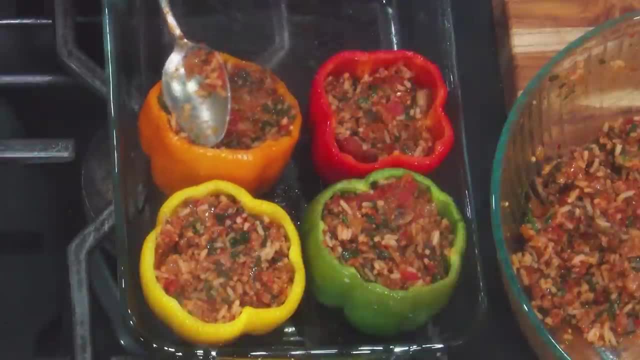 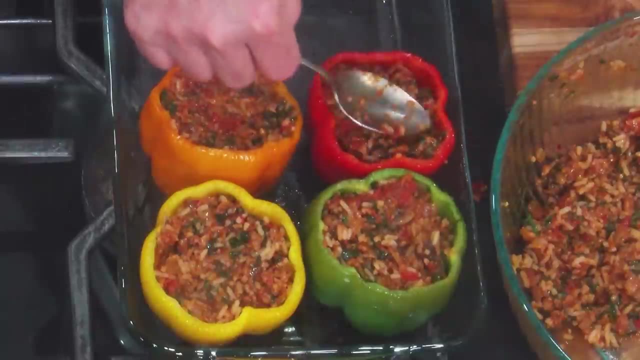 Don't be afraid to push it in. Okay, You want it to be really, really, really full? See the way I'm doing it. I'm really like: not enough, Not much left. I love it when I have extra left. 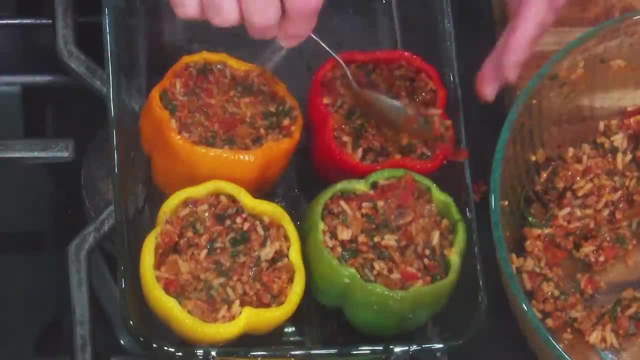 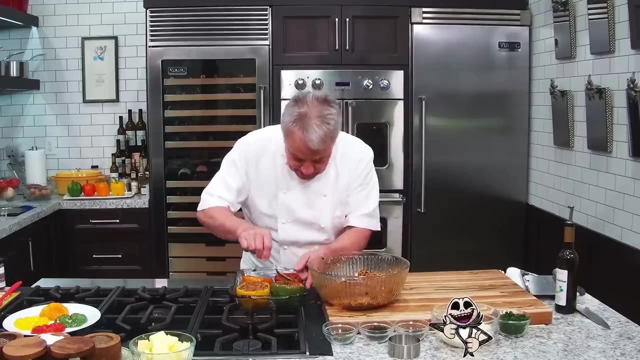 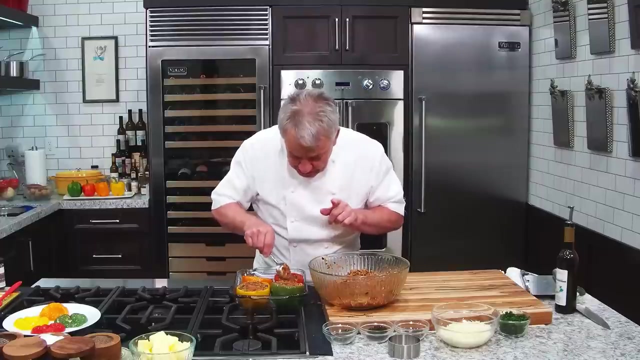 Because I eat it just like this. Forget about stuffing the rest of the peppers, I eat it just like this. Now, some people- Jack is one of them- He mixes the cheese with all that stuff. Nothing wrong with that. My opinion is, the cheese overwhelms everything. 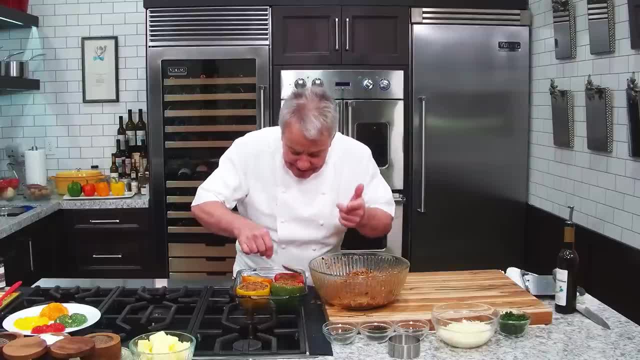 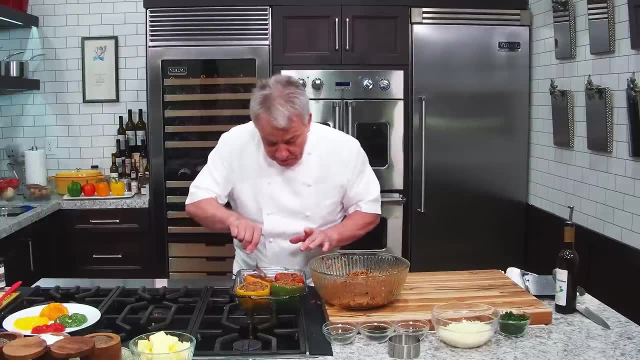 Then all of a sudden you don't taste the delicacy of the sausage and all that stuff, Because the cheese overwhelms everything. It just does. So it's up to you if you want to put the cheese inside. Try my way one time. 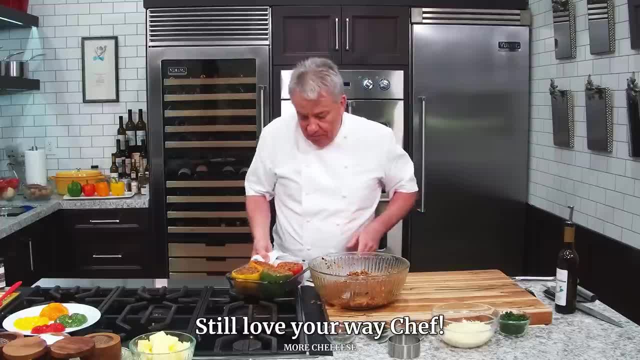 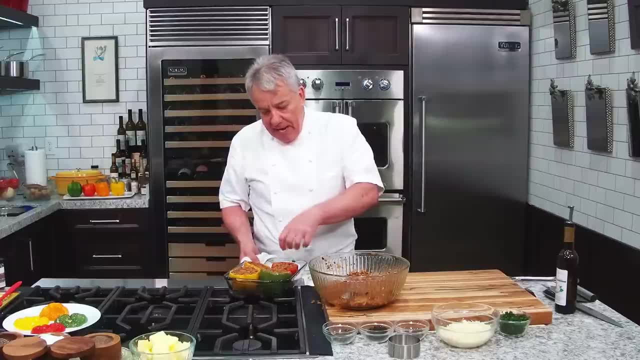 And you may keep doing it this way. It's really up to you. I pop this in the oven, I'm going to cook them another 25 minutes And then I'll come back. We'll put the cheese And then we'll take them out. 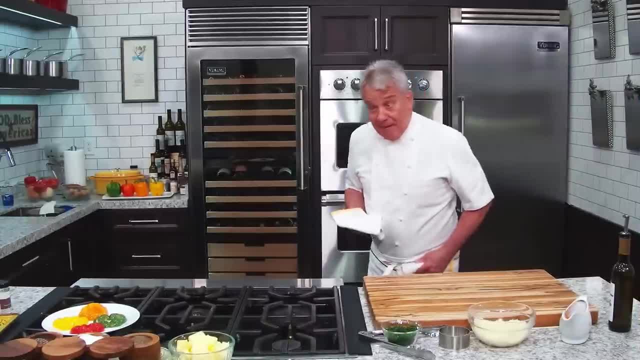 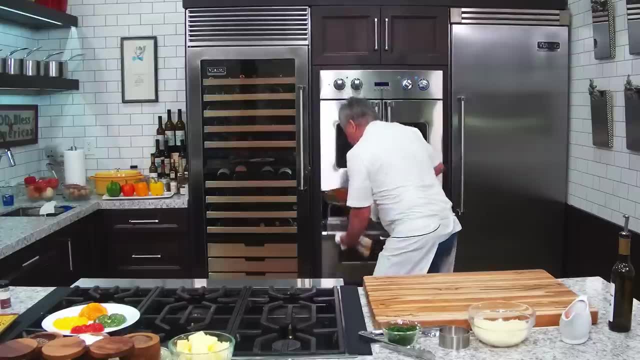 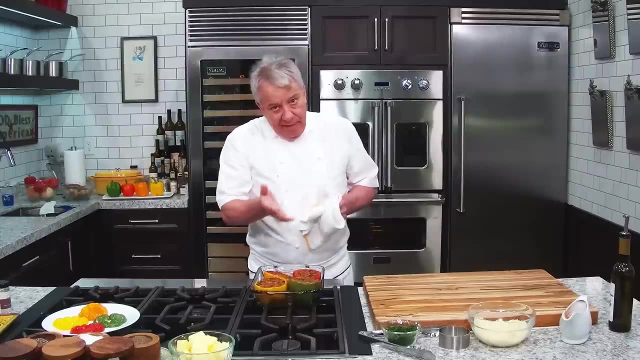 Be back in a few minutes. Okay, Let's take them out of the oven, friends, Let's take them out, And they're going to be hot, And so it depends how thick they are and how thin they are. You can get away with 15, 20 minutes. 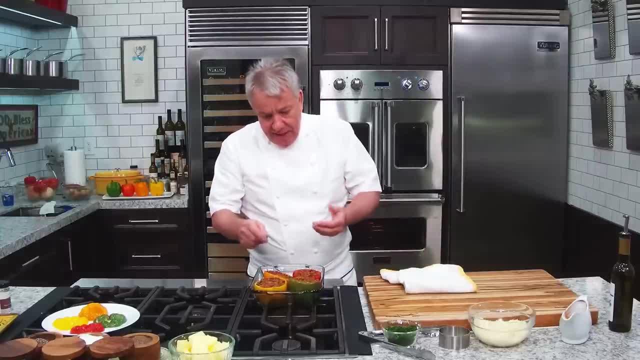 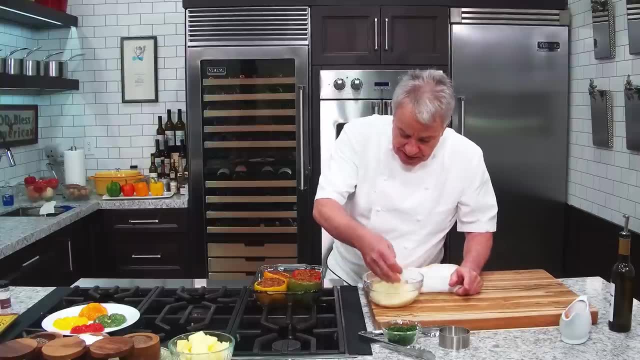 Okay, It's really up to you. It all depends how thin they are, Because if they're thin, you see like those guys are going to be ready soon. So what I got to do is I'm going to put some cheese in there. 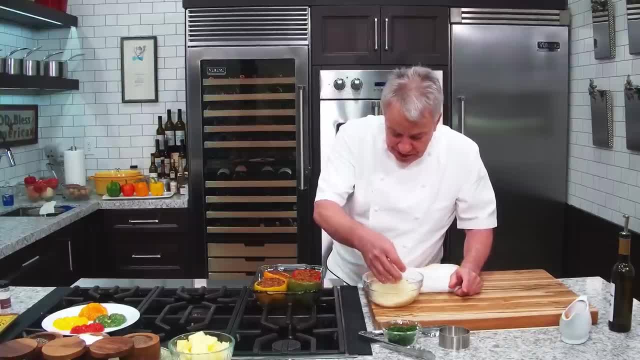 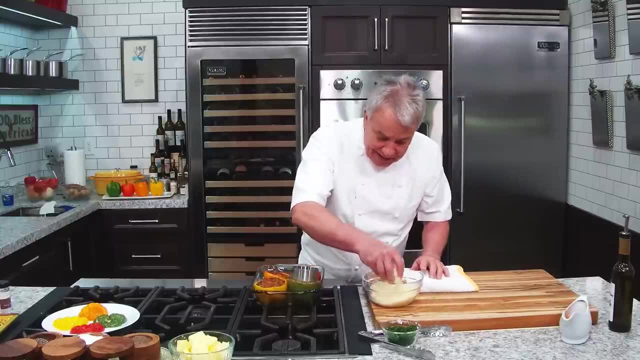 You can put cheddar cheese, You can put gruyere cheese, You can put mozzarella cheese, jack cheese, Put whatever cheese you want in here. friends, Just to try to make it nice, I'm just going to go like this. 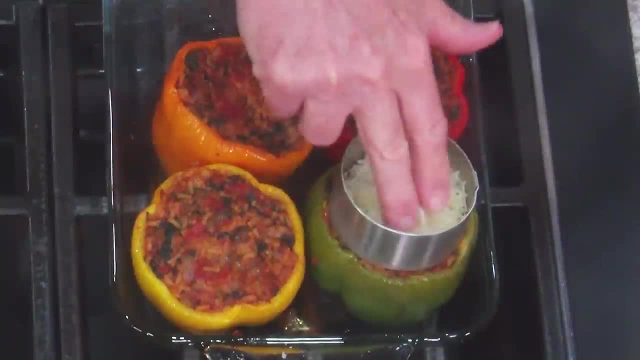 And we want to be generous, But some people like to put it all over the place. It's really up to you how you want it. You know I like to be nice. You know clean When I put my cheese in it. 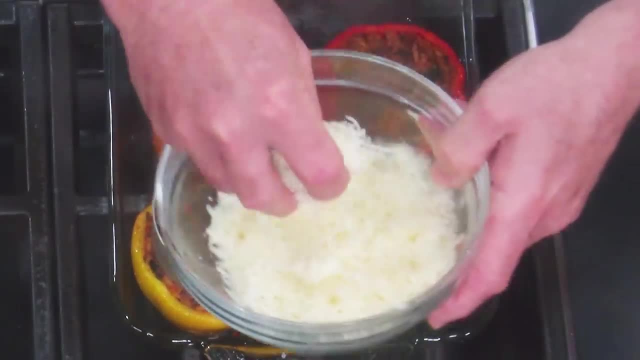 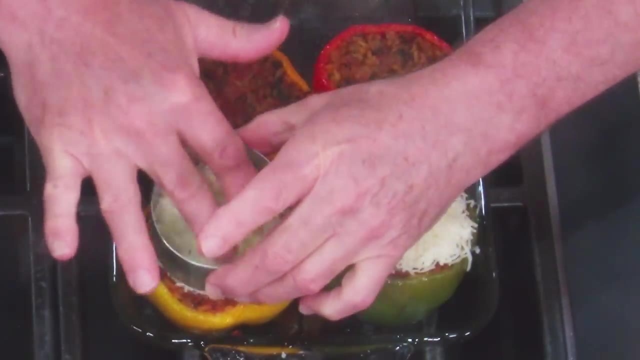 So it's really up to you how you put it in there, my friends. Okay, Some people just like to slab it all over the place, And there's nothing wrong with that If it makes you happy to do it this way. 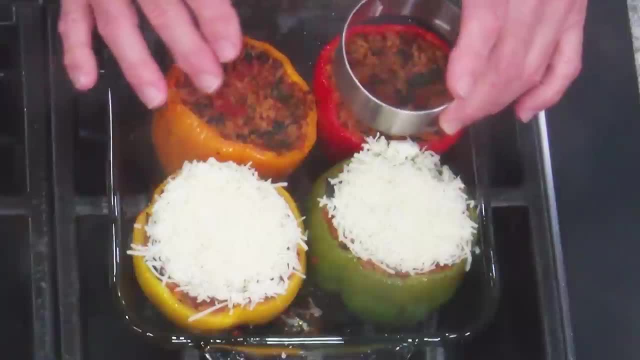 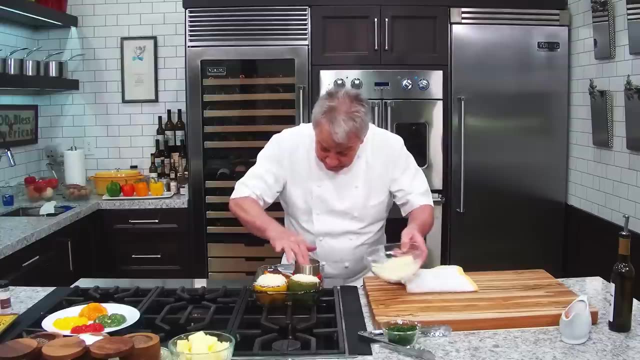 See, take it out. I think you have enough right here. It's not too slappy, But it's okay. It's going to be delicious, no matter what we do, my friends. So, like I said, you can put the cheese mixed with a mixture if you want. 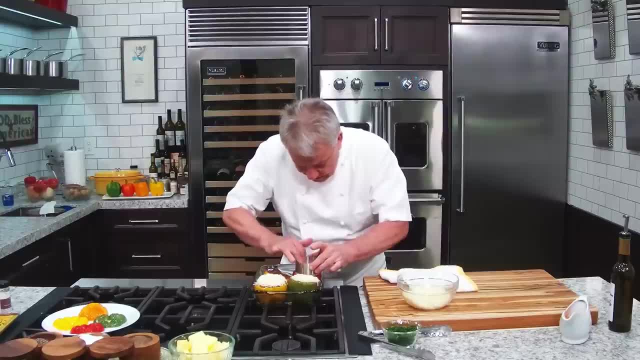 But I tell you what I think it's: It's better that way, Just like this. It's up to you, Of course. it's up to you. It's always up to you, friends, Forget about what we do, chefs. 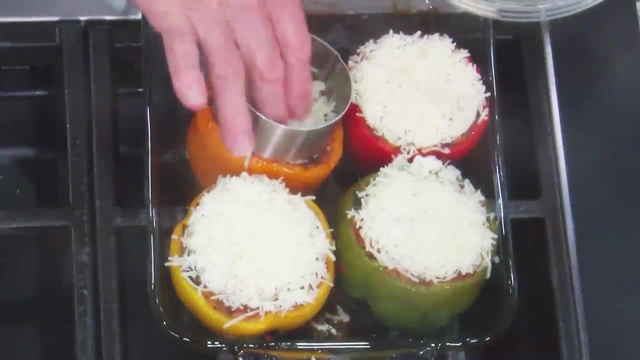 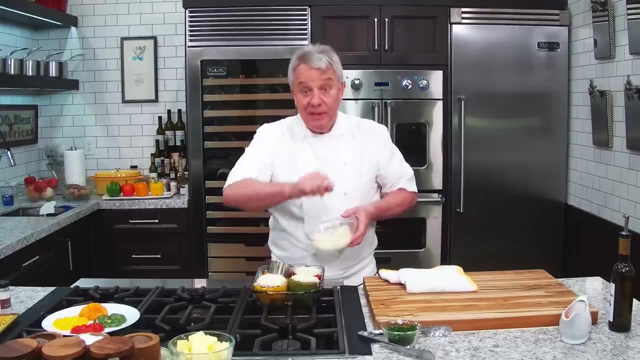 We're just here to show you our technique, But you know, you make it your own. It's your home, your family, your cook, however you want it. There's no right or wrong here. Your right is what you decide. 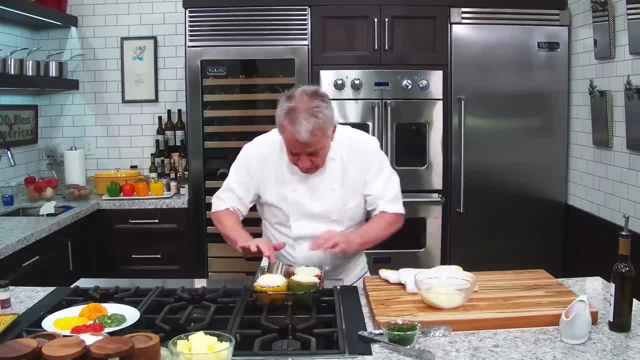 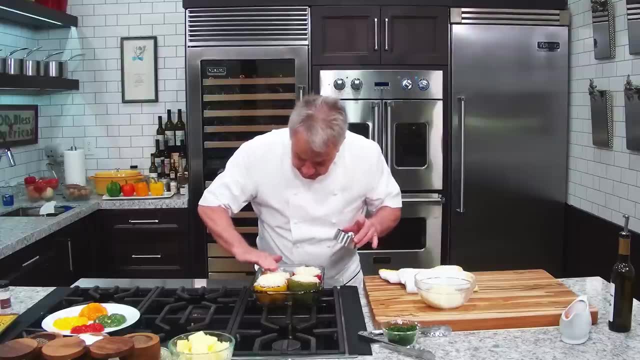 That's what it's all about, friends, Not about what I decide, What you decide. All right, And here we have it. We're just going to take it And we're just going to pop them in the oven until the cheese is nicely melted. 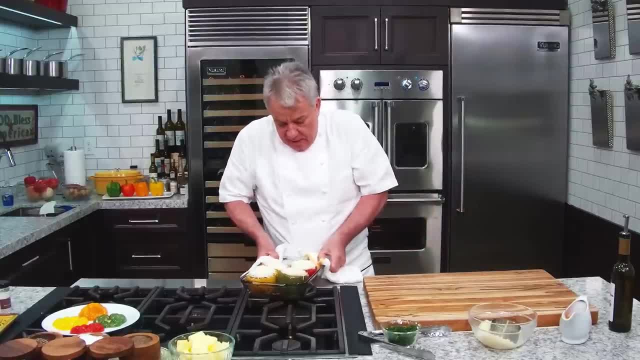 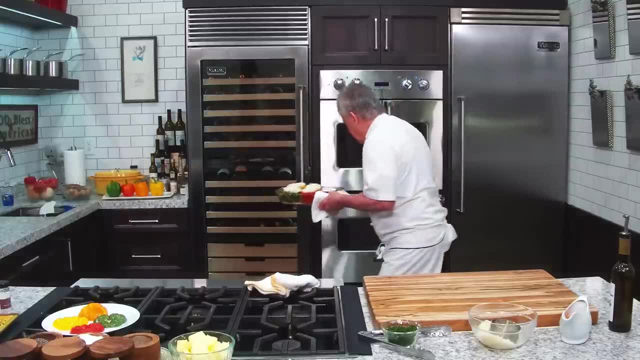 So we'll be back in a few seconds. One a few seconds. However long it takes to get a golden brown, It depends on your oven, It depends on everything. So we're going to wait a little bit, friends, All right. 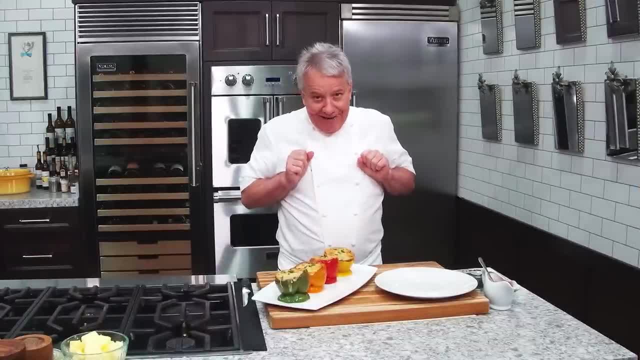 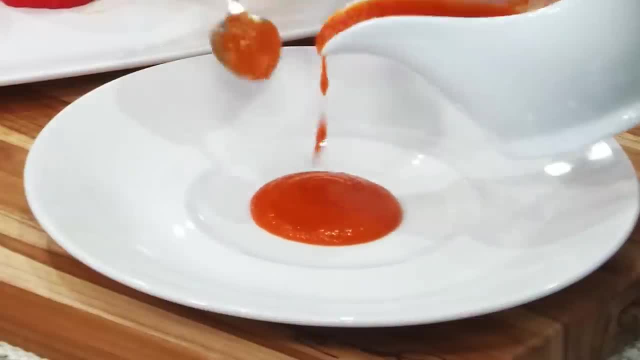 I'll be back in a few minutes. Okay, friends, I'm ready to eat now And I'm hungry. I'm going to serve it with a bell pepper coulis. You know I make that sauce. There's a video on it. 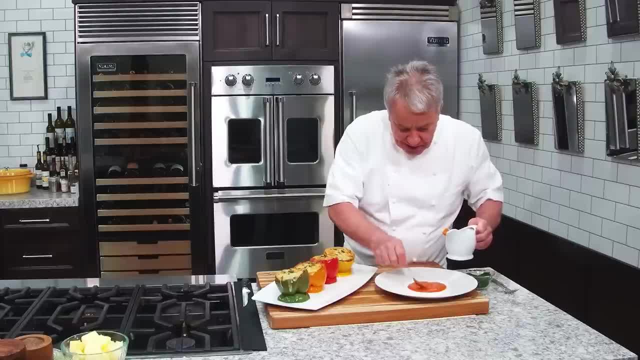 This is an old video. This was in an old kitchen. You guys got to check it out. This is so simple to make. You're not going to believe it, friends. You got to make this up. The recipe is over there somewhere. 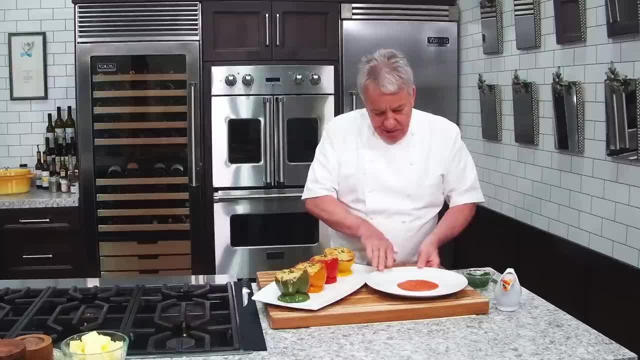 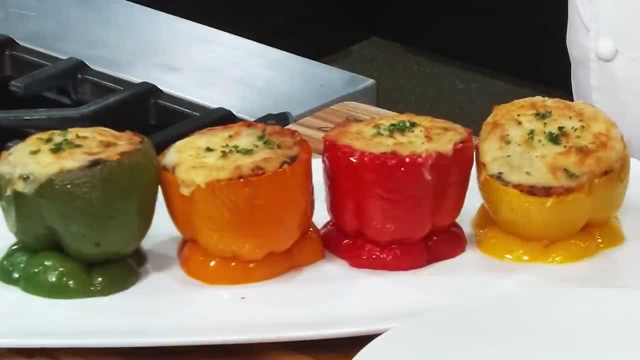 I think it's over there And you got to try to make that. It's really cool, So we're going to plate it. You see what I did. I took the top. put it on the bottom as a stand, if you will. 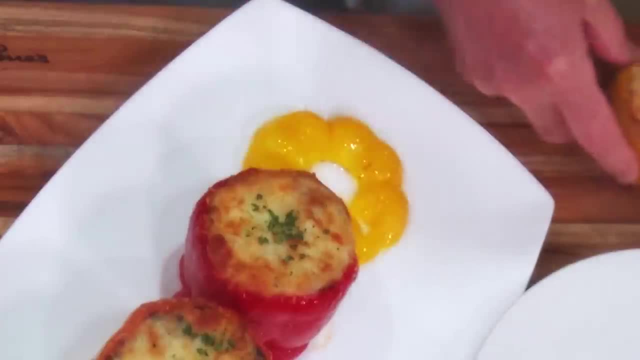 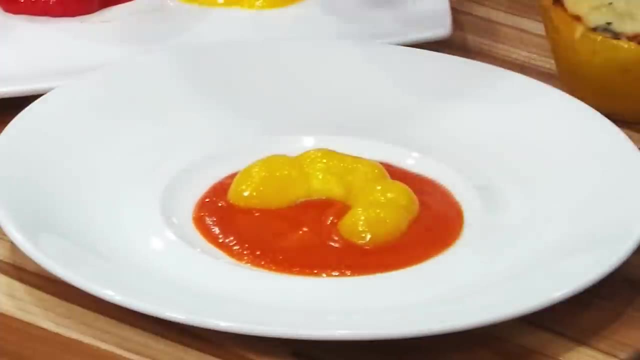 Matter of fact, remember, the one in the yellow is broken. So you see what we're going to do: We're going to take it. You see, it doesn't matter if it's broken, Take it If it's in broken pieces. this one ended up breaking in two or three pieces. 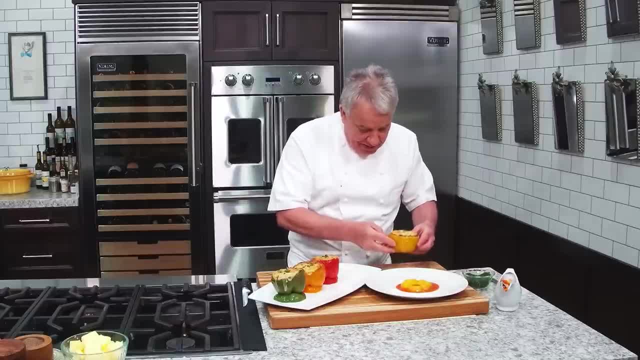 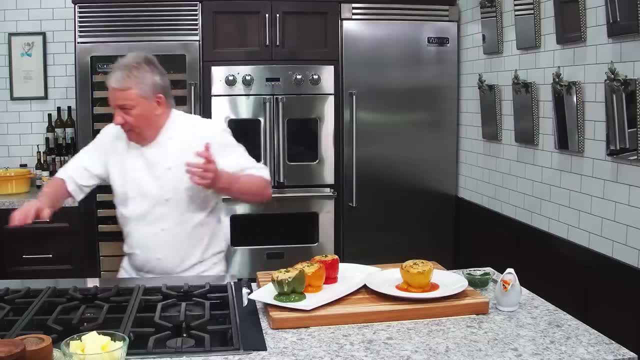 It doesn't matter, This is a stand. And now what we're going to do? we're going to put it up And hopefully for you, it's going to stand. It's beautiful. You see, my friend, It's a beautiful presentation, isn't it? 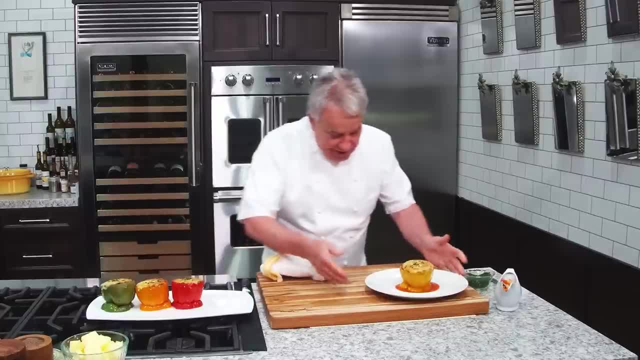 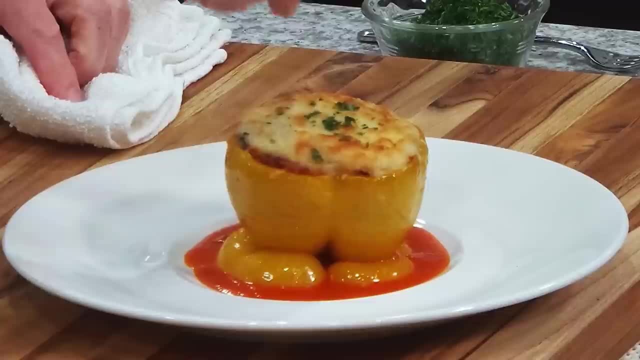 So let me just take it out of the way. All of a sudden, roasted bell pepper can have a little class, And there's no reason It should not have a little class. right, A little chopped parsley in there, friends. 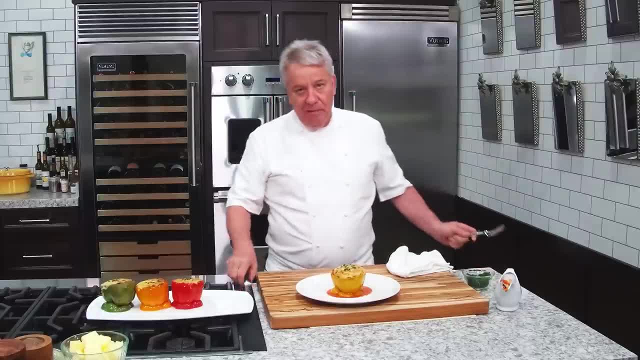 And then what we're going to do, we're going to eat it. That's the best moment. I waited a little bit because otherwise I'm going to burn myself. I do that a lot. So what we're going to do, we're going to go in there, friends. 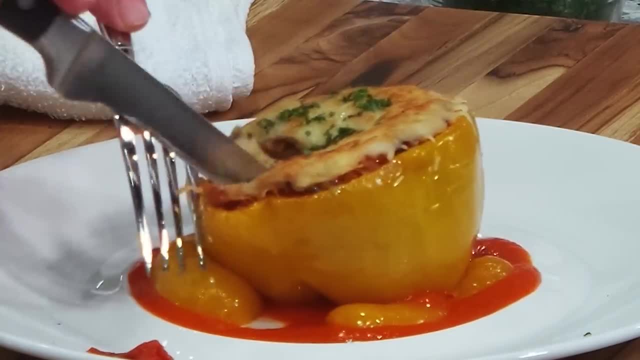 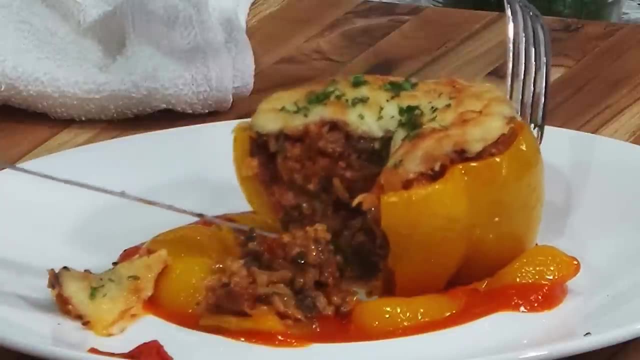 And we're going to cut. And let me tell you, friends, You're probably not going to be able to see much because I'm not being very generous with the camera, But I think you can see a little bit in there. And this right there, let me tell you: 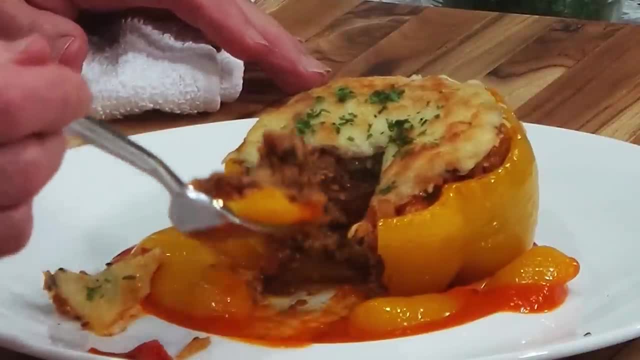 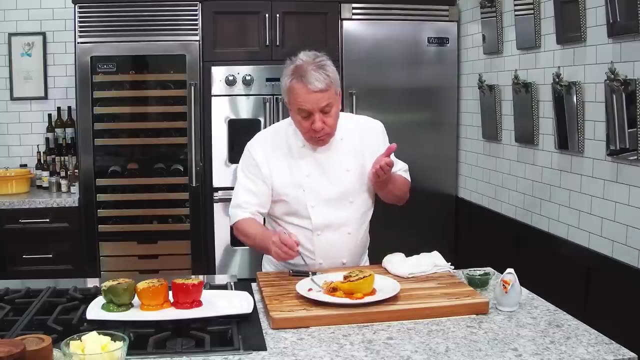 This is going to be Amazing. It's still a little hot, though. I can see some smoke coming out of there, So it's still going to be delicious. Why don't I take a big bite like this, Mmm?